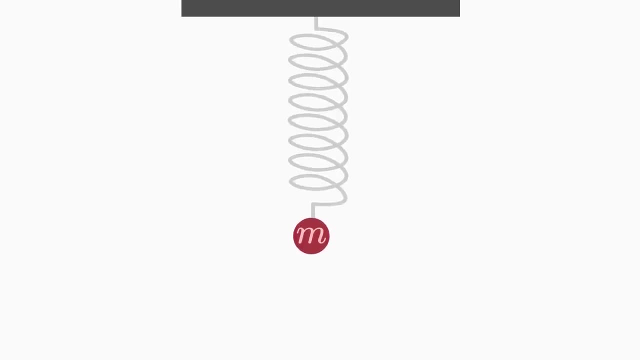 and release it, the spring will start swinging back and forth Without friction, as in this case, it will never stop swinging. While the mass oscillates, the displacement Y changes. The displacement is therefore dependent on the time t, Thus also the acceleration A depends. 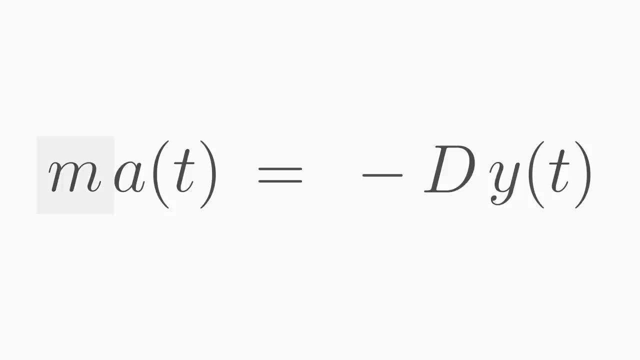 on the time t. The mass, of course remains the same at any time, no matter how much the spring is displaced. This is also true in good approximation for the spring constant D. If we now look at the mass of the spring, we can see that the mass of the spring is the same at any time, no matter how much the spring is displaced. This is also true in good approximation for the spring constant D. 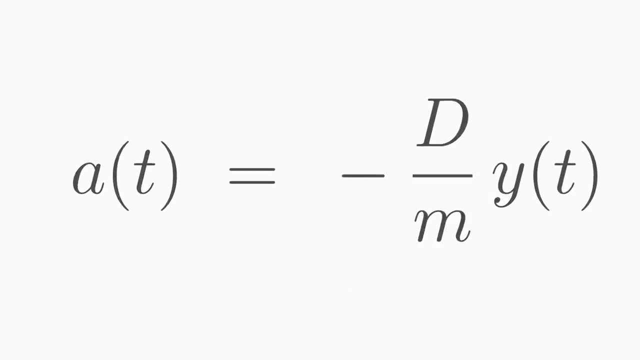 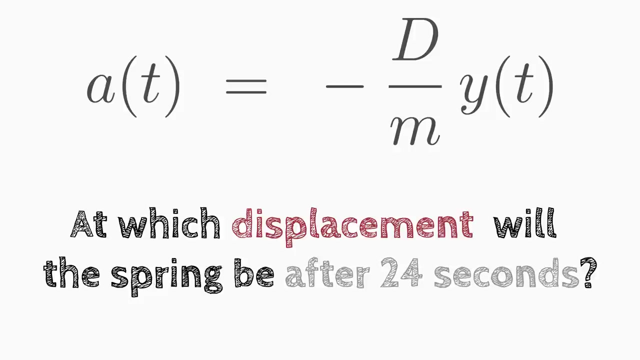 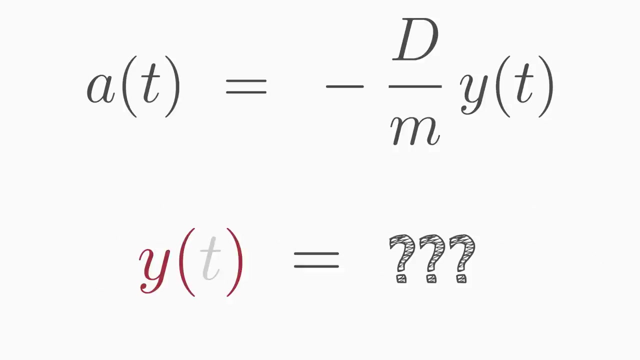 If we now bring M to the other side, we can use this equation to calculate the acceleration experienced by the mass at each displacement Y. But what if we are interested in the question at which displacement Y will the spring be after 24 seconds? To be able to answer such a future question, we must know how exactly Y depends on the time t. We only know 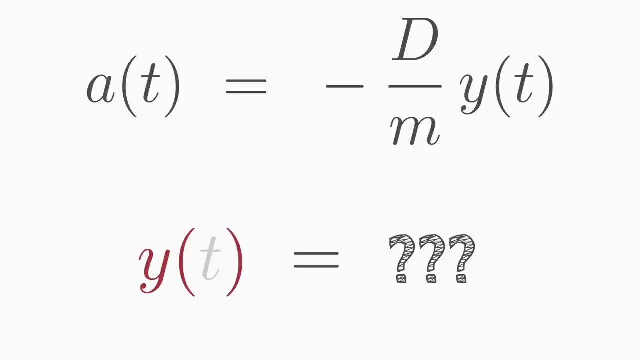 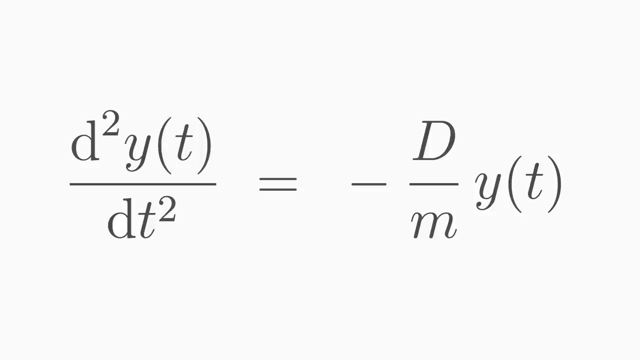 that Y DOES depend on time, but not how And exactly. when dealing with such future questions, differential equations come into play. We can easily show that the acceleration A is the second time derivative of the distance traveled, so in our case it is the second derivative of Y. 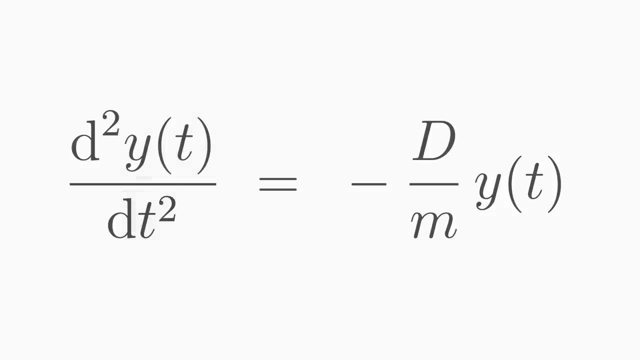 with respect to time t. Now we have set up a differential equation for the displacement Y. You can recognize a differential equation, in short DEQ, by the fact that, in addition to the surged function Y, it also contains derivatives of this function, like in this case, the second. 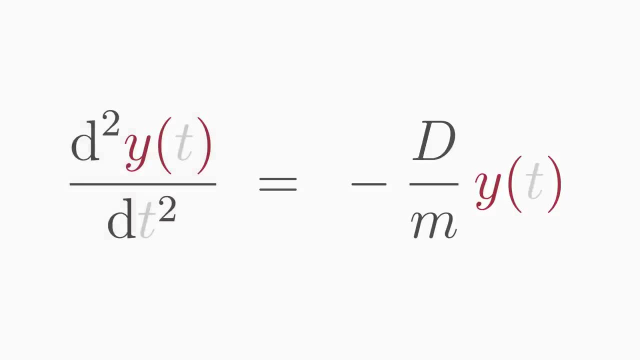 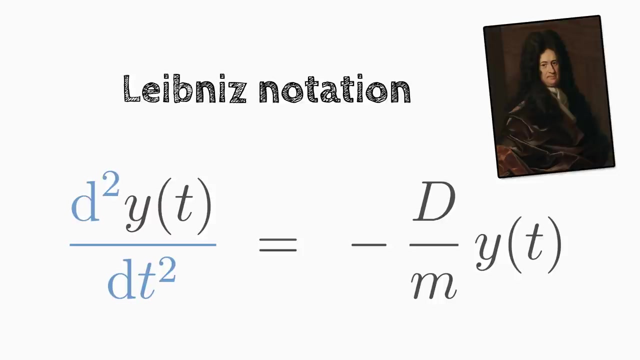 derivative of Y with respect to time t. A differential equation is an equation containing a surged function, Y, and derivatives of this function. You will certainly encounter a many notations of a differential equation. We have written down our differential equation in the so-called Leibniz notation. You will often encounter this notation in physics. We can also 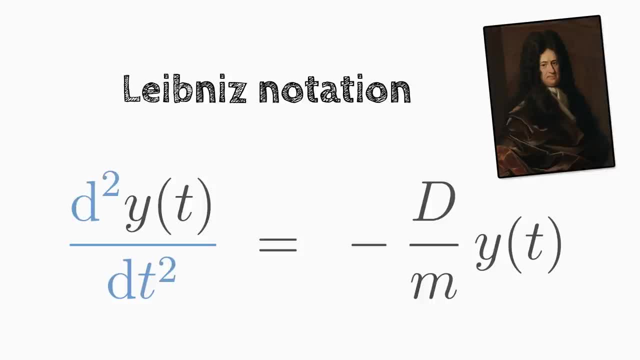 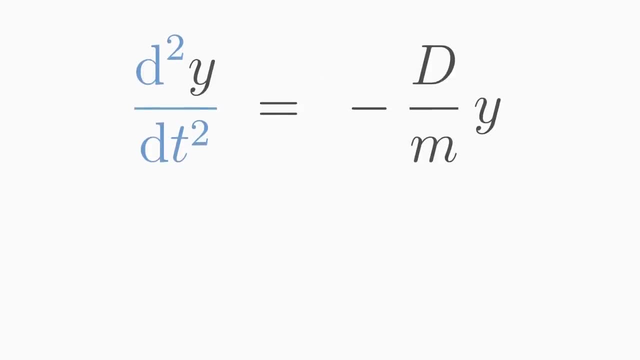 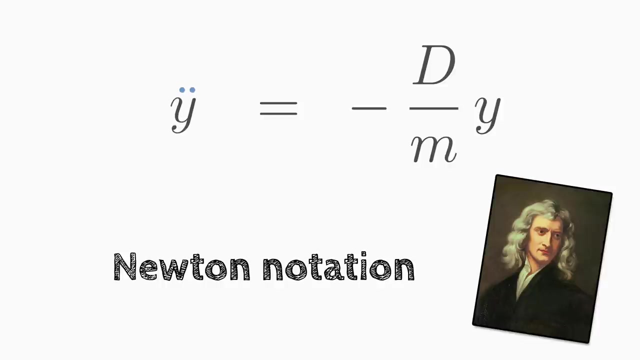 write it down a bit more compactly without mentioning the time dependence. If the function Y depends only on the time t, then we can write down the time derivative even more compactly with the so-called Newton's equation: One time derivative of Y corresponds to one point above Y, so if there is a second time derivative, 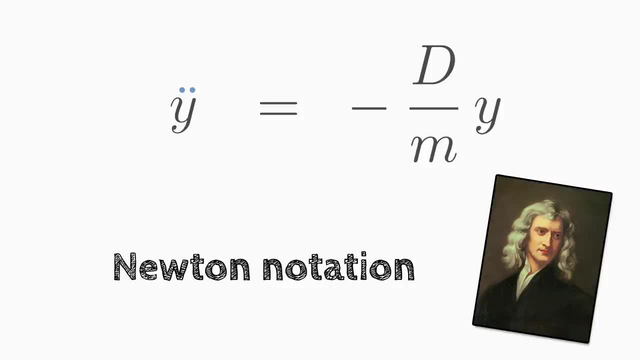 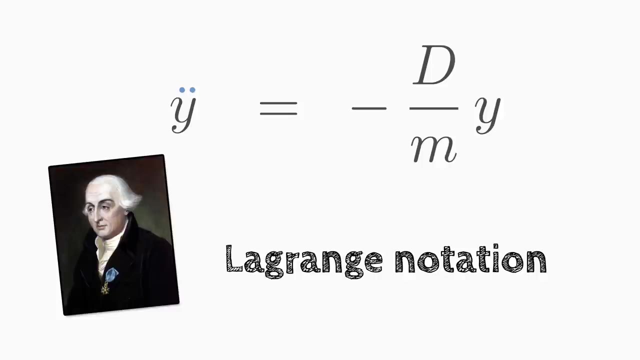 as in our case, there will be two points. Obviously, this notation is rather unsuitable if you want to consider the tenth derivative, for example. Another notation you are more likely to encounter in mathematics is the Lagrange notation. Here we use primes for the derivatives. 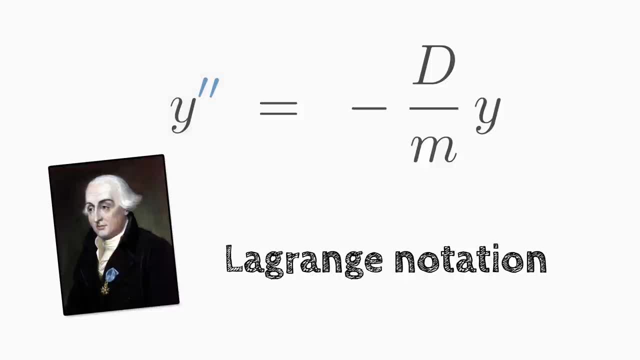 So for the second derivative, two primes In Lagrange notation it should be clear from the context with respect to which variable the function is differentiated. If it is not clear, then you should write out explicitly on which variables Y depends. Each notation has its. 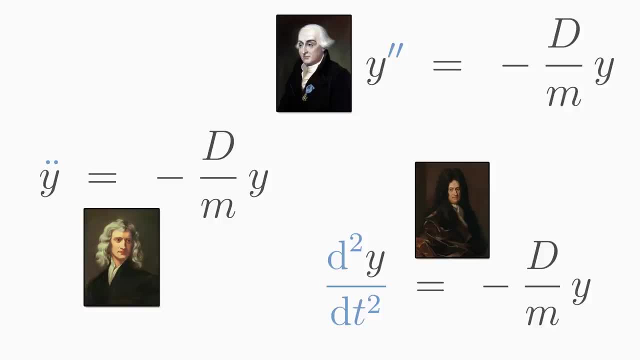 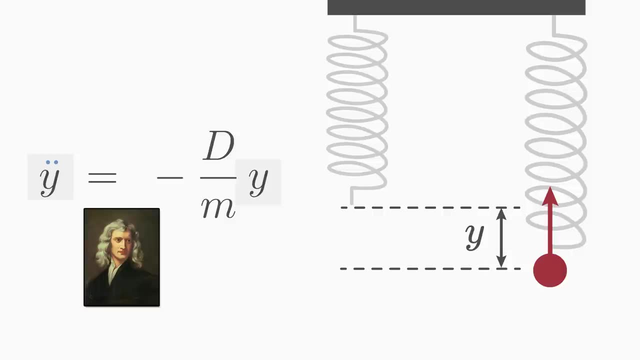 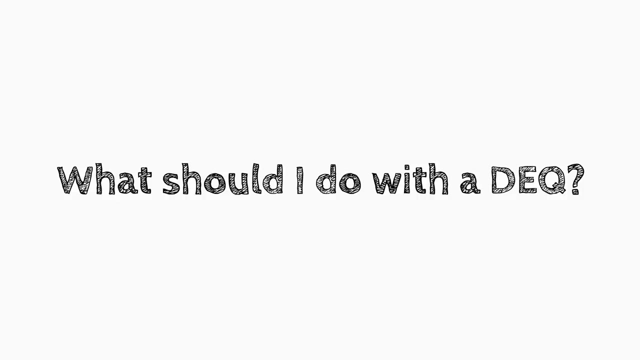 advantages and disadvantages. However, remember that these are just different ways of writing down the same physics. Even rearranging and renaming does not change the physics under the hood of this differential equation. To answer our previous question: at which displacement Y will the spring be after? 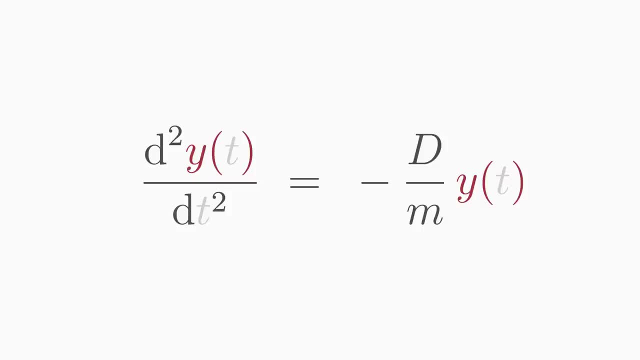 24 seconds. we must solve the post-differential equation. Solving a differential equation means that you have to find out how the function Y you are looking for exactly depends on the variable T. For simple differential equations, like the one of the oscillating mass, 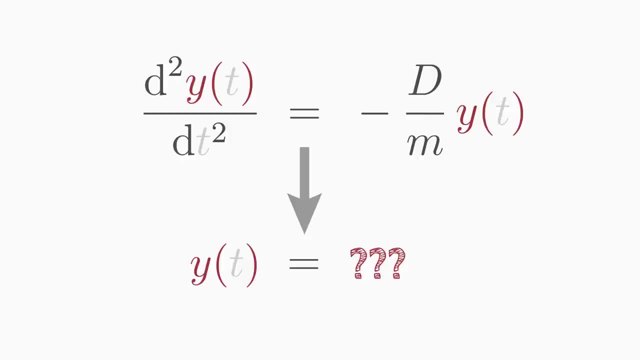 there are solving methods you can use to find the function Y. Keep in mind, however, that there is no general recipe for how you can solve an arbitrary differential equation. For some differential equations there is not even an analytic solution. Here the word analytic means that you cannot write down a concrete equation for the function Y, The 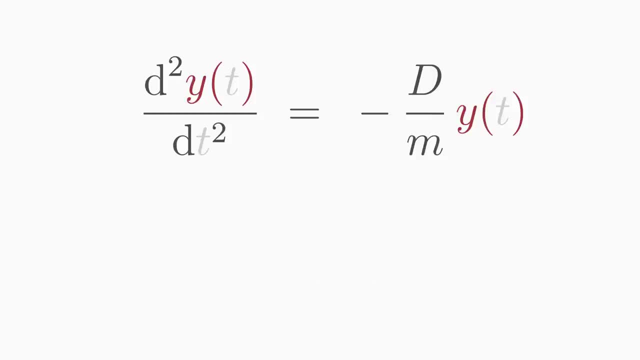 only way to solve the differential equation is to find the function Y. However, if you can't solve the function Y, the only possibility in this case is to solve the differential equation on the computer numerically. Then the computer does not spit out a concrete formula, but data points which you can 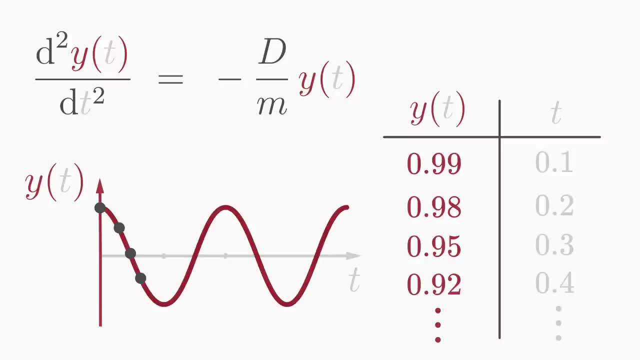 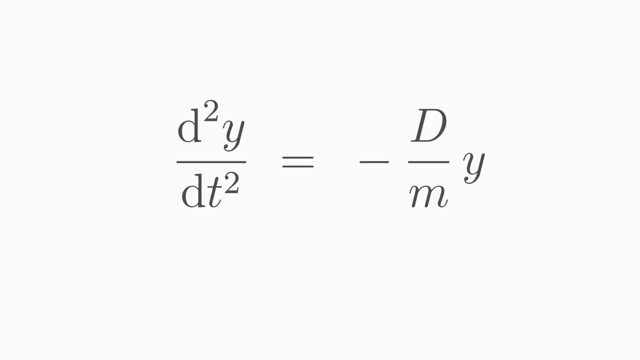 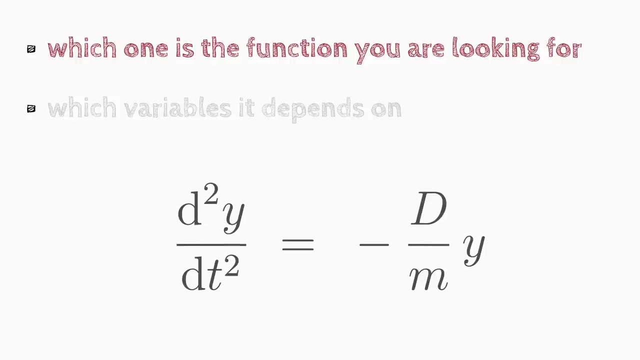 represent in a diagram and then analyze the behavior of the differential equation. Once you encounter a differential equation, the first thing you need to figure out is which one is the function you are looking for and which variable it depends on. In our differential equation of the oscillating mass, 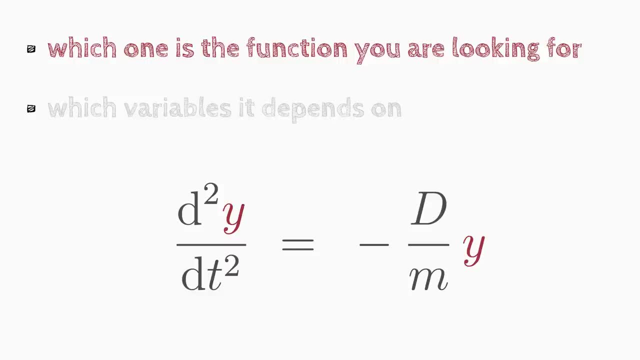 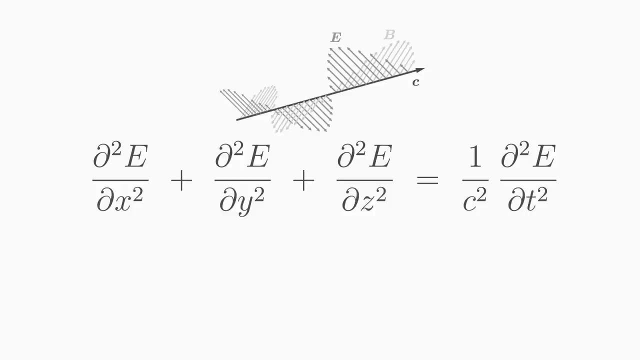 the function we are looking for is called Y and it depends on the variable T. As another example, look at the wave function that describes the electric field of an electromagnetic wave propagating at the speed of light c. What is the function you are looking for in this differential equation? It is the function E, because its derivatives occur here. 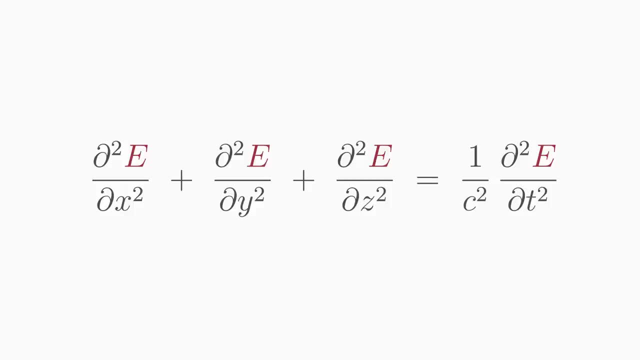 On which variable does the function E depend? The dependence is not explicitly given here, but from the derivatives you can immediately see that E must depend on X, Y, Z and on T, That is, on a total of four variables. Let's look at a slightly more complex example. This system of differential equations describes: 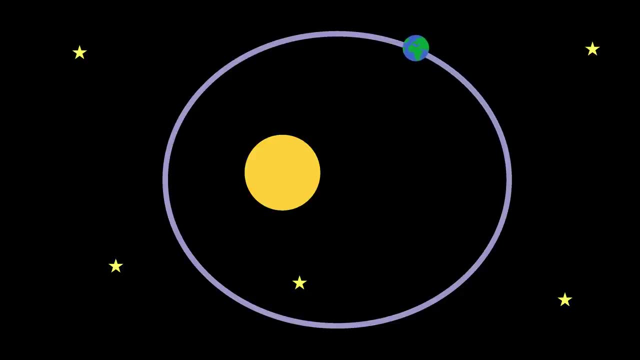 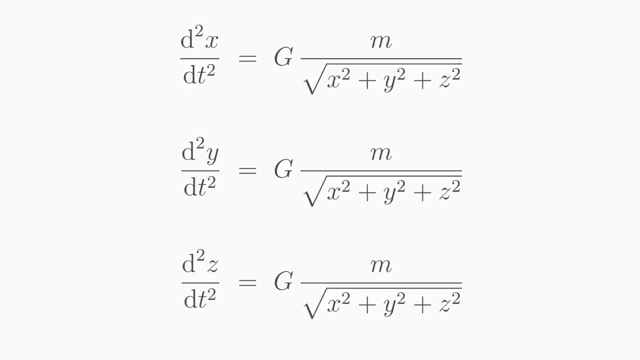 how a mass moves in a three-dimensional gravitational field. Here you have a so-called coupled differential equation system. In this case, a single differential equation is not sufficient to describe the motion of a mass in the gravitational field. In fact, three functions are searched here, namely the trajectories X, Y and Z. 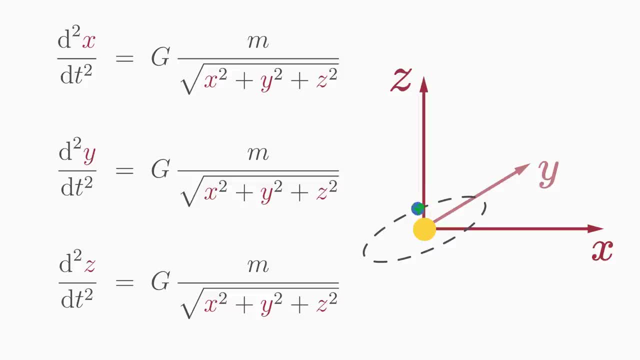 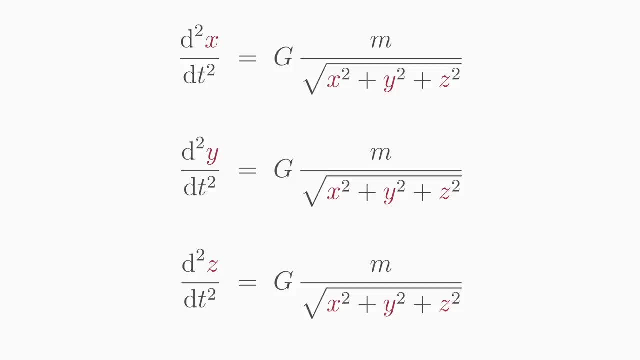 which determine a position of the mass in three-dimensional space. Each function describes the motion in one of the three spatial directions And all three trajectories only on the time t. What does it even mean if we have coupled differential equations? The word coupled means that, for example, in the first differential equation for the function x, 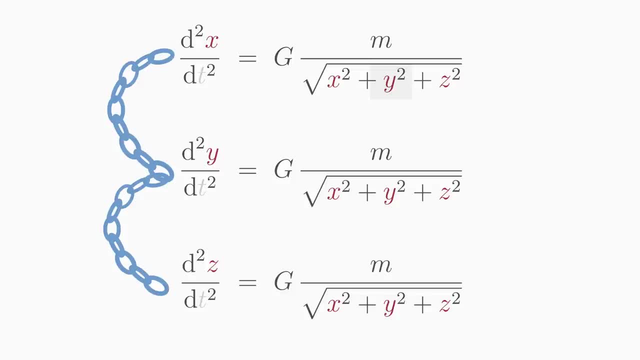 there is also the function y. So we cannot simply solve the first differential equation independently of the second one, because the second equation tells us how y behaves in the first equation. In all three differential equations, all of the searched function, x, y and z, 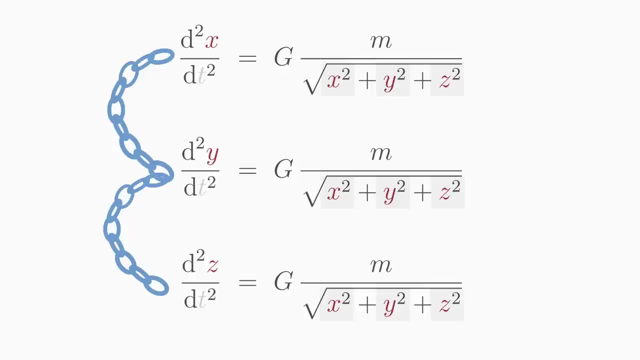 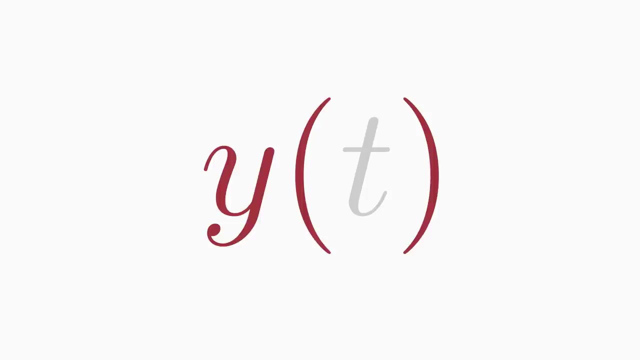 occur, which means that we have to solve all three differential equations simultaneously. After you have found out what function you are searching for and which variables it depends on, you should answer some more basic questions to get to know the differential equation better. Is the differential equation ordinary? 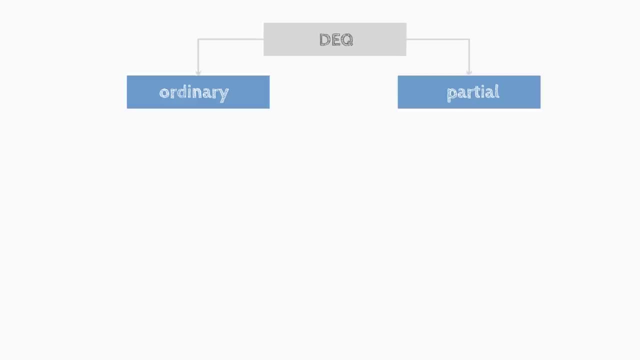 Or partial. Partial differential equations describe multidimensional problems and are significantly more complex. Of which order is the differential equation? First-order differential equations are usually easy to solve and describe, for example, exponential behavior such as radioactive decay or the cooling of a liquid. Differential equations. 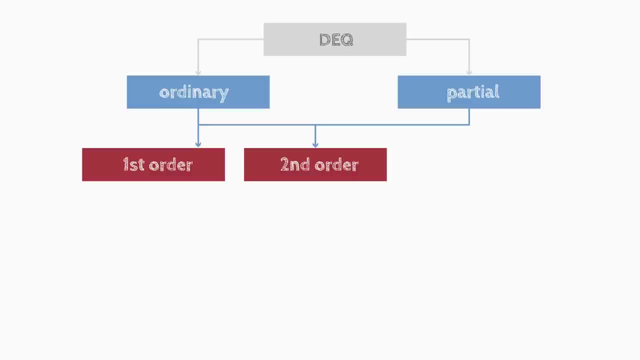 of second order, on the other hand, are somewhat more complex and also often occur in nature. Maxwell's equations of electrodynamics, Schrödinger's equation of quantum mechanics, these are all second-order differential equations. Only starting from the second order, a differential 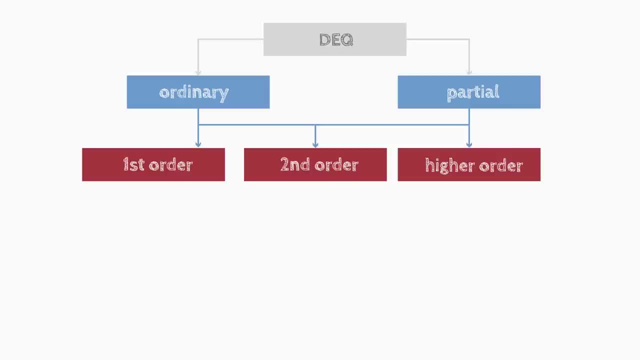 equation can describe an oscillation, And only starting from the third order a differential equation can describe chaos. Is the differential equation linear or non-linear? The superposition principle applies to linear differential equations. The superposition principle applies to linear equations, which is incredibly useful, for example, in the description of electromagnetic. 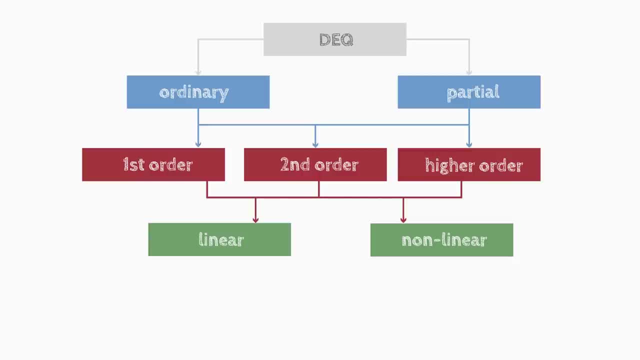 phenomena. Nonlinear differential equations are much more complex and occur, for example, in nonlinear electronics, in the description of superconducting currents. Moreover, chaos can only occur in nonlinear differential equations of third order and higher. When you encounter such an equation, sometimes the only thing you can do is throw away your pen and paper. 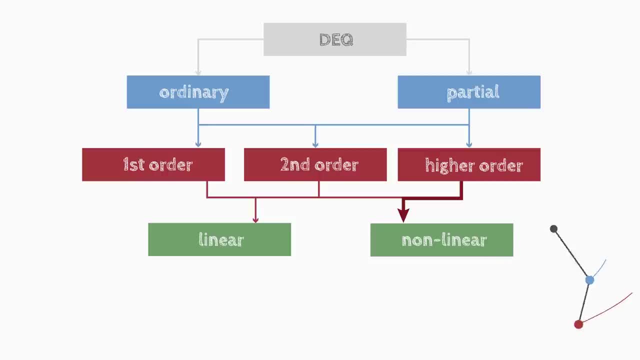 and solve the equation numerically on the computer. Many nonlinear differential equations cannot even be solved analytically. Is the linear differential equation homogeneous or inhomogeneous? Homogeneous linear differential equations are simpler than inhomogeneous ones and describe, for example, an undisturbed oscillation, while inhomogeneous 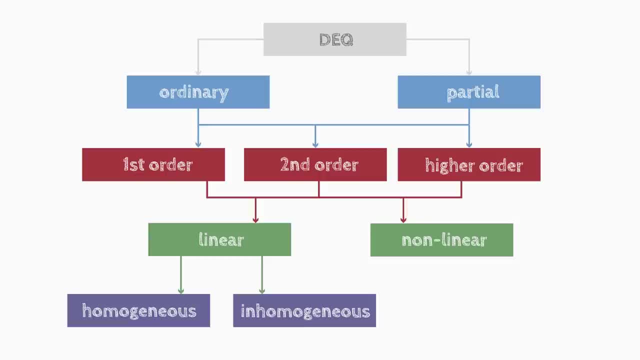 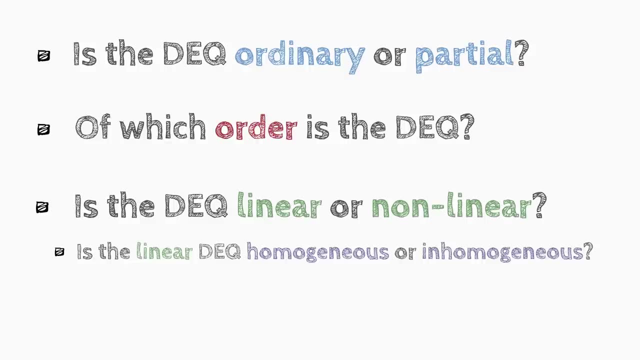 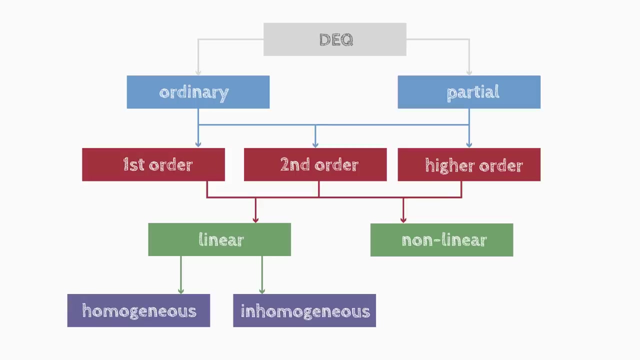 differential equations are also able to describe externally disturbed oscillations. First, let's learn how to answer these questions. After you have classified a differential equation, you can then specifically apply an appropriate method to solve the equation. Even if there is no specific solving method, you will know how complex a differential equation is based on the 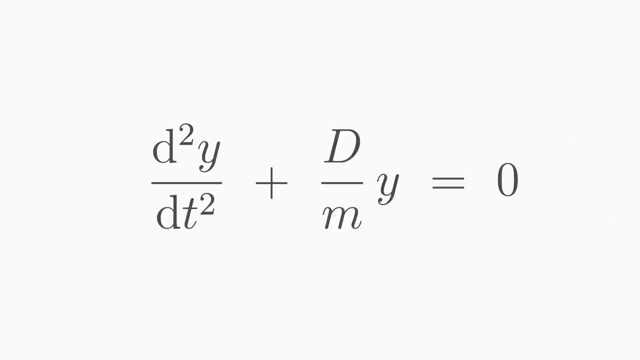 classification. Our equation for the linear differential equation is the one that we will use to solve the equation on the substituted version of the oscillating mass, so that it is semblantly linear instead of beingассediable like in the previous example. 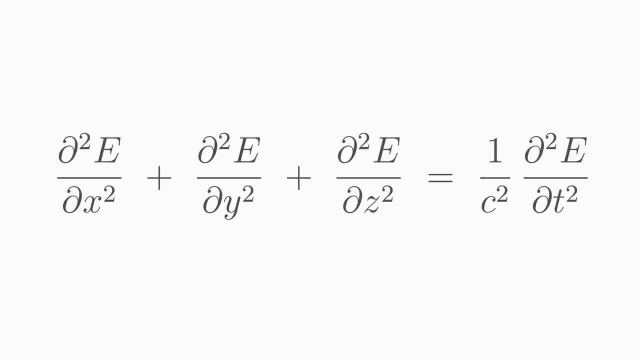 In this case on the time t. The wave equation, on the other hand, is a partial differential equation. Partial means that the surged e function depends on at least two variables, and derivatives with respect to these variables occur in the equation. the equation, In this case e, depends on four variables: t, x, y and z- and in the differential, 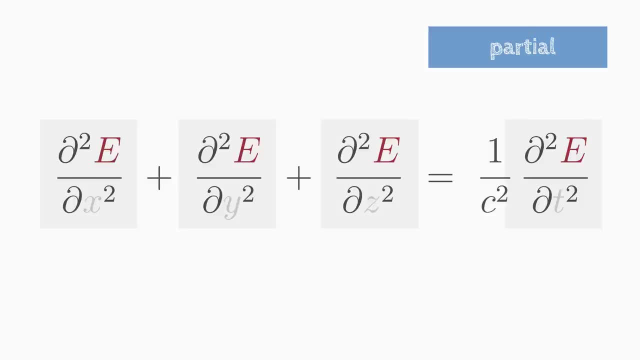 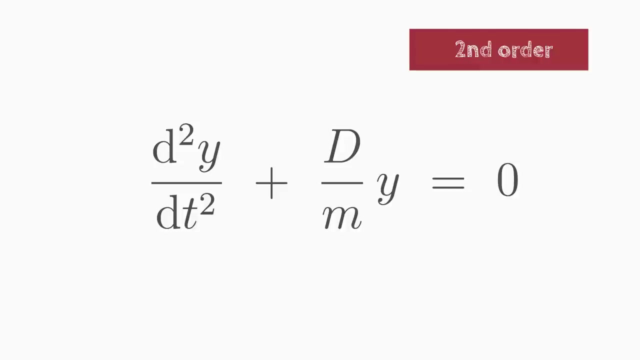 equation also, derivatives with respect to t, x, y, z appear. Furthermore, our equation for the oscillating mass is a differential equation of second order. The order of the differential equation is the highest occurring derivative of the searched function, Since in our equation the 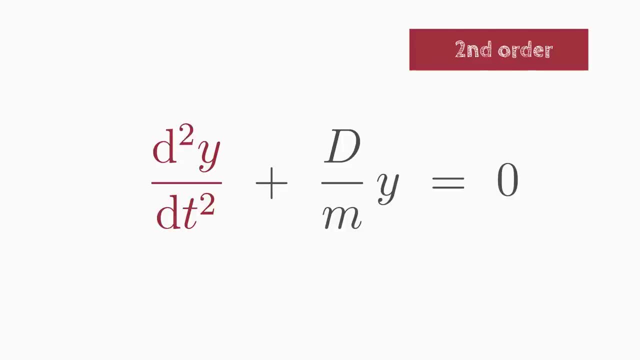 second derivative of y is the highest one. this is therefore the second-order differential equation. The differential equation for the radioactive decay law, on the other hand, is a first-order differential equation, because the highest occurring derivative of the searched function, n, is the first derivative. Moreover, our equation for the oscillating mass is linear Linear means. 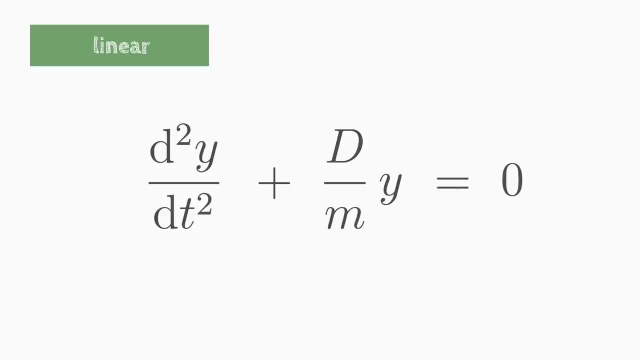 that the searched function and its derivative are the same. Similarly, the second derivative of x is the second-order derivative of y. What are the properties of the derivate, of the derivative? The derivatives here contain only powers of one and there occur no products of derivatives. 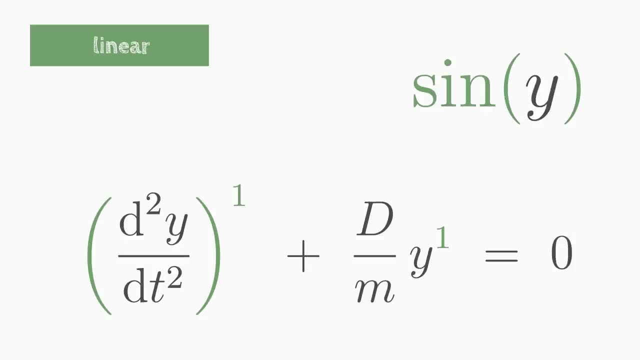 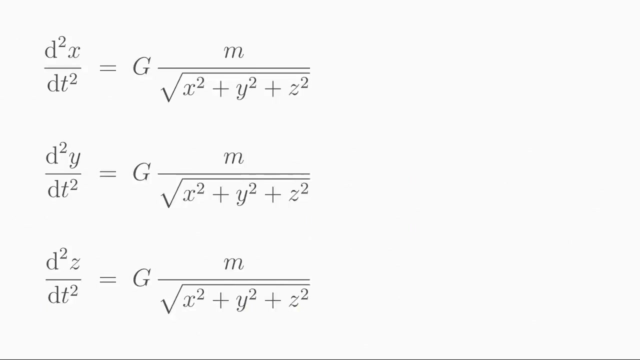 with the function, like y squared or y times the second derivative of y. There also occur no composed functions like sine of y or square root of y, second derivative. The radioactive decay law is also linear. What about the wave equation? It is also linear. The coupled differential equation system for the motion of a mass and 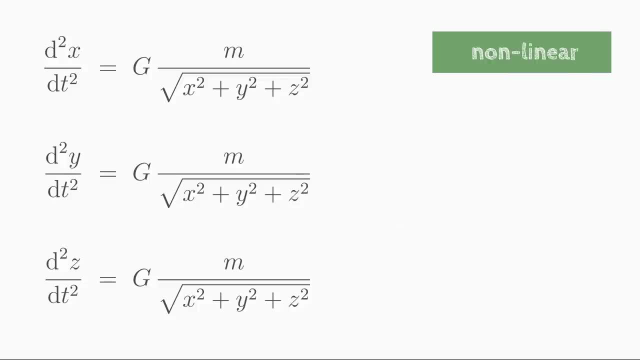 a gravitational field, on the other hand, is nonlinear. Here the search functions x, y and z occur in quadratic form. But even if the squares were not there, there would still be the square root and the fraction, which make the differential equation system nonlinear. 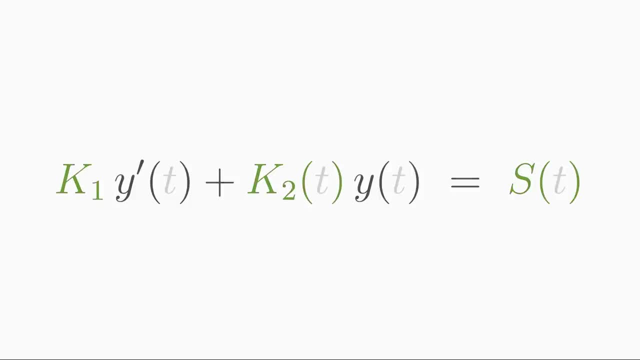 In the next types of differential equations, the coefficients multiplied by the search function and its derivatives are important In some solving methods. it is important to distinguish between constant coefficients and non-constant coefficients. Constant coefficients do not depend on the variables on which the search function depends. Non-constant coefficients. 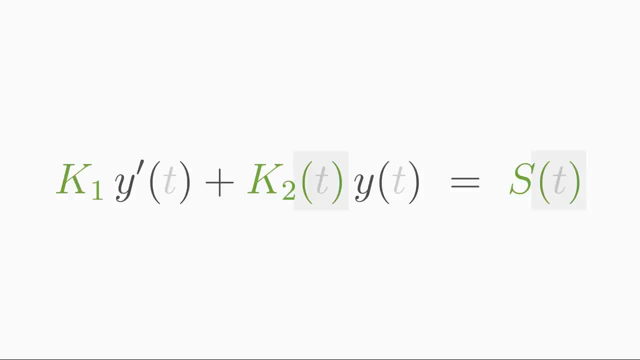 do depend on the variables on which the search function depends. A coefficient must not necessarily be multiplied with the search function or its derivative. It can also stand alone. In this case we call the single coefficient a perturbation function. In our differential equation for the oscillating mass there is a constant coefficient. 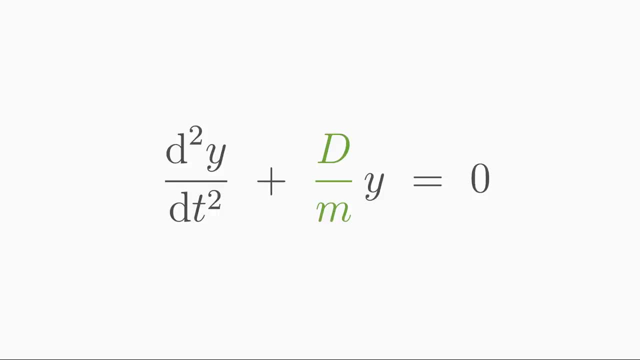 which is multiplied by the search function y, namely d over m. Strictly speaking. the search function y is a constant coefficient which is multiplied by the search function y, namely d over m, Strictly speaking. there is also a coefficient in front of the second derivative, namely 1,. 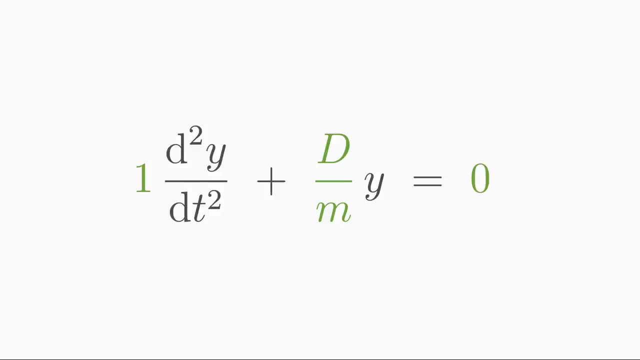 and the single coefficient, that is the perturbation function, is zero here, so it does not exist. If the perturbation function is zero, then we call the linear differential equation homogeneous. So the differential equation for the oscillating mass is a homogeneous differential equation. 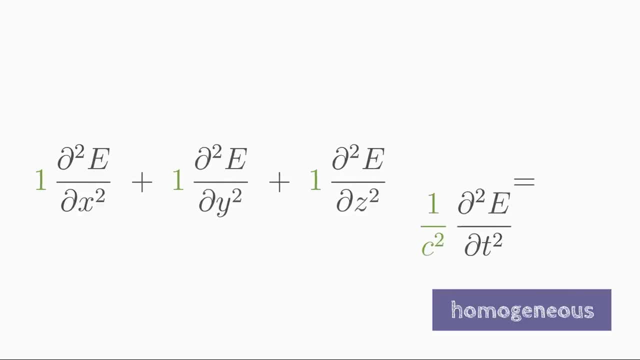 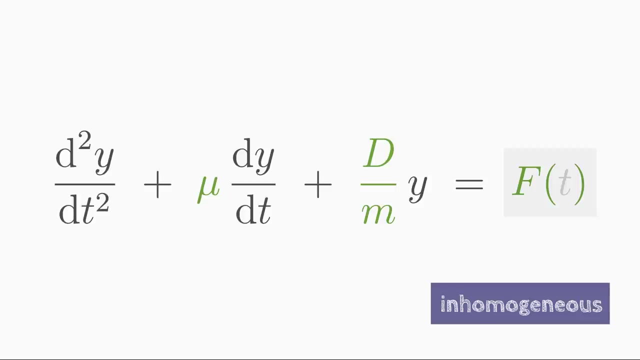 The wave equation is also homogeneous, Because here there is also no single coefficient. The perturbation function is zero. The differential equation for a forced oscillation, on the other hand, is inhomogeneous. Here the external force f corresponds to the perturbation function. 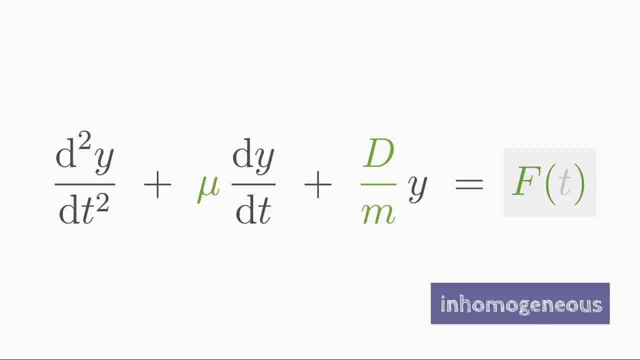 As you can see, it stands alone, without being multiplied by the function y or its derivatives. Moreover, the perturbation function f is time-dependent, so it is a non-constant coefficient. A differential equation alone is not sufficient to describe a physical system uniquely. 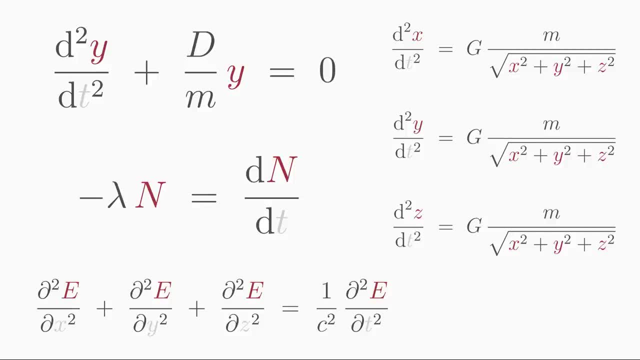 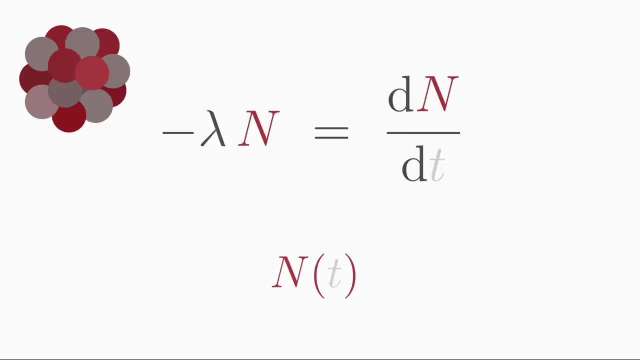 The solution of a differential equation describes quite a few possible systems that have a certain behavior. For example, the solution of the radioactive decay law describes an exponential behavior. However, the knowledge about an exponential behavior is not sufficient to be able to say concretely how many atomic nuclei have decayed, for example, after 10 seconds. 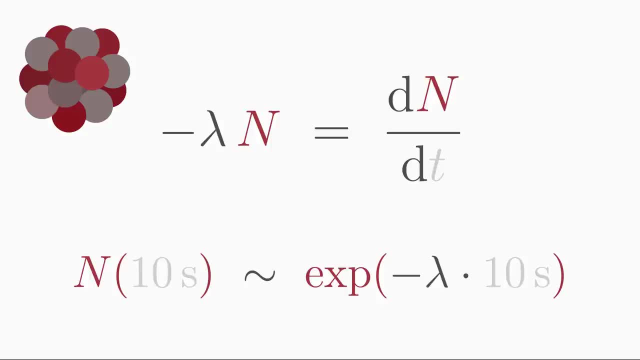 This is exactly why, for every differential equation, there are usually given constraints. These are additional information which must be given to a differential equation in order to specify the solution of the equation. The number of necessary constraints depends on the order of the differential equation. 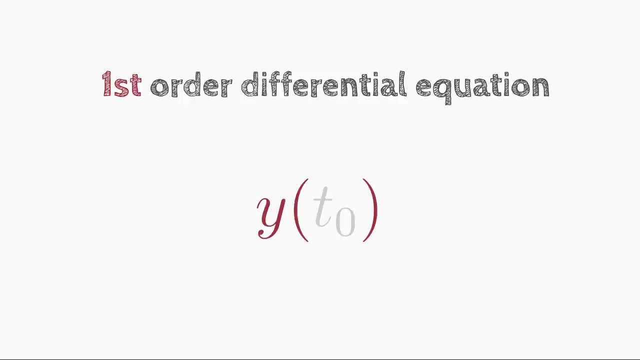 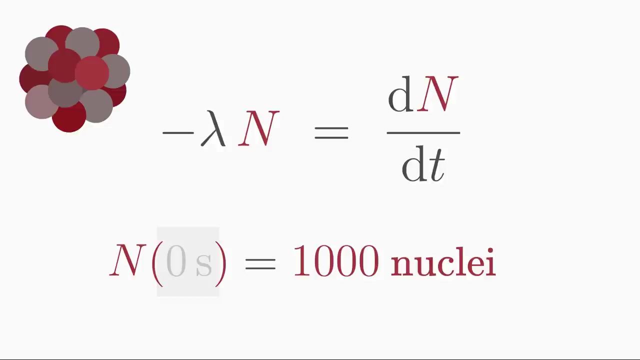 For a first-order differential equation a single constraint is necessary, namely a function value of the searched function. For the radioactive decay law, for example, it should be stated how many not-yet-decayed atomic nuclei were present at the time. t equals zero. 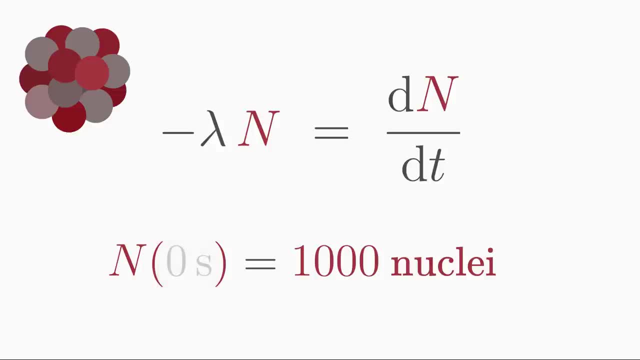 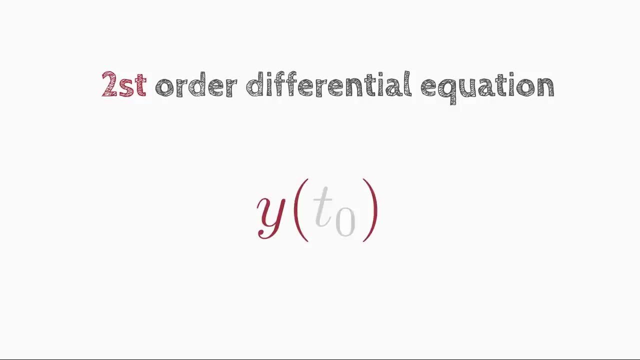 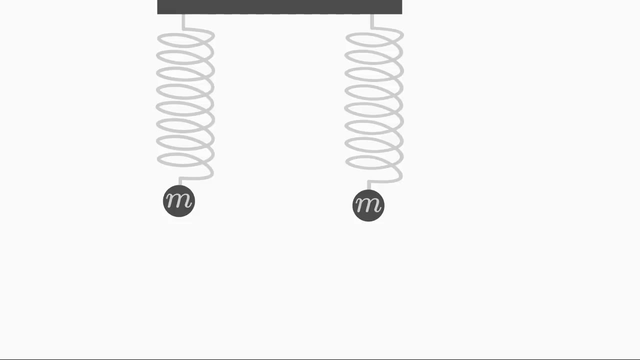 For example, 1000 atomic nuclei at time, t equals zero. For a second-order differential equation, two constraints are necessary: A function value of the searched function and, for example, a function value of the first derivative. For an oscillating mass, the function value could be y of zero equals one. 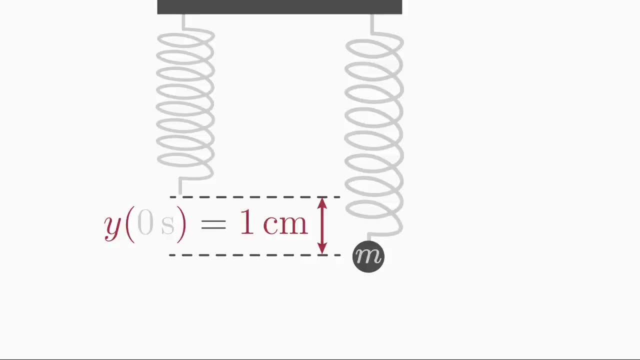 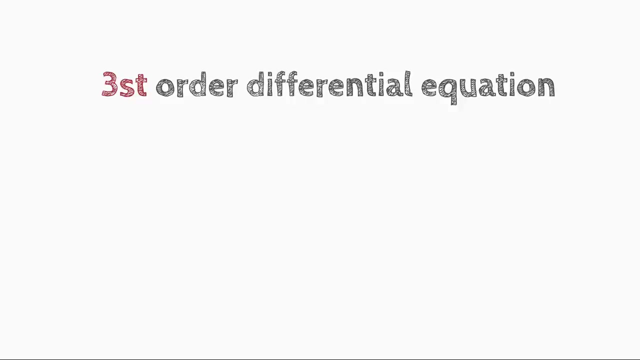 which sets the initial displacement to one at time, zero And the function value of the first derivative, that is, the velocity, could be: y prime of zero is equal to zero, which sets the initial velocity of the mass For a third-order differential equation. 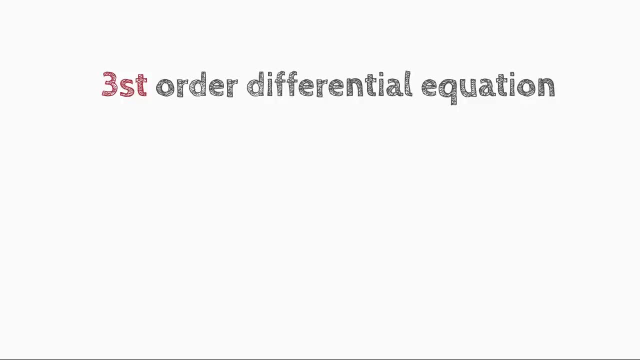 then three constraints would be necessary to describe a system uniquely: A function value of the searched function, a function value, for example, of its first derivative and a function value, for example, of its second derivative For a fourth-order differential equation. 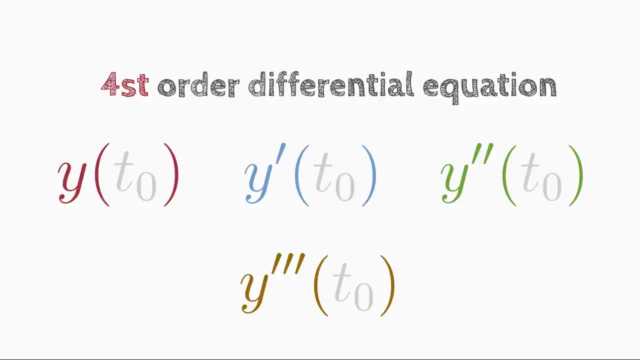 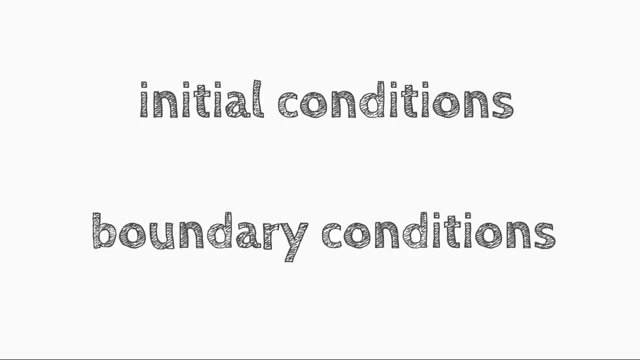 then four constraints would be necessary, and so on. Most of the time, you will come across the so-called initial conditions and boundary conditions. These are just names for constraints that tell you what kind of information you have about the system. Sometimes, for example, you know in which state the system was at a certain time. 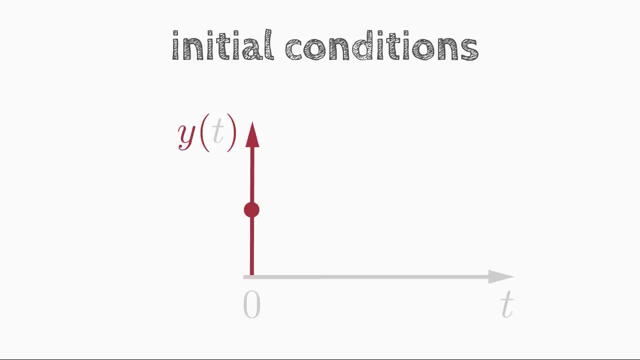 This could be the initial time at which you displaced and released the mass on a spring. You specify at one certain point in time, for example, at time t equals zero, which value the displacement y had. And since we need two constraints, we need to know which value the displacement y had. 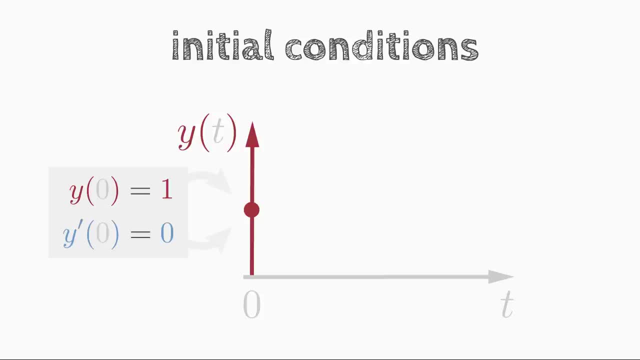 And since we need two constraints for the oscillating mass, you also specify which value. the derivative y prime, that is, the velocity had at the same point in time. t equals zero. In such a case we speak of initial conditions. We call a differential equation, together with initial conditions, an initial value problem. 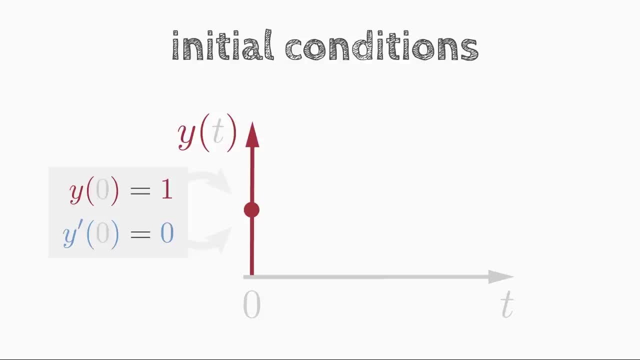 If we solve the initial value problem, we can use the solution to predict the future behavior of the system. Sometimes you are unlucky and do not know the velocity of the oscillating mass at a certain initial time, So you don't know the derivative y prime at time zero. 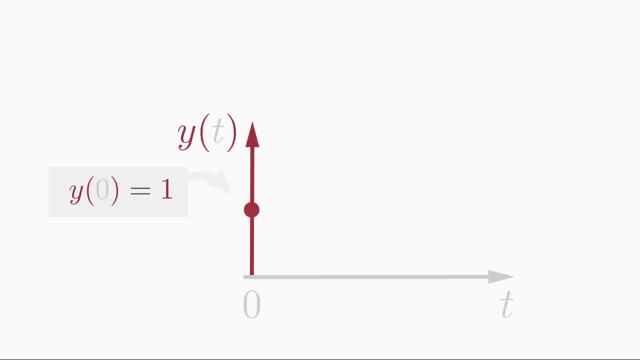 at which you also know the displacement y. But you really need two constraints, otherwise you can't calculate concrete numbers. But maybe you know that, for example, after 6 seconds the oscillating mass was in the maximum displaced state. If you have constraints given to describe the system at two. 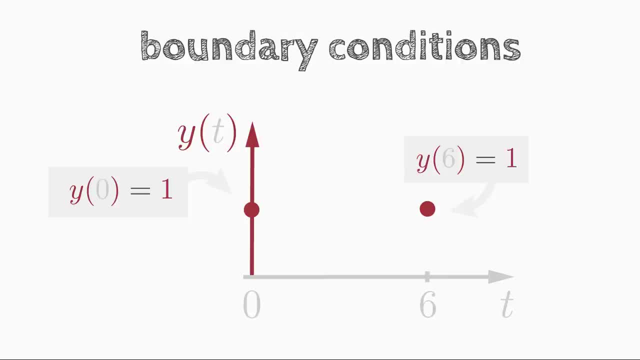 different points in time, then we call them boundary conditions. We call a differential equation together with two or more boundary conditions a boundary value problem. If we solve the boundary value problem, we can use the solution to predict how the system behaves within these boundaries. 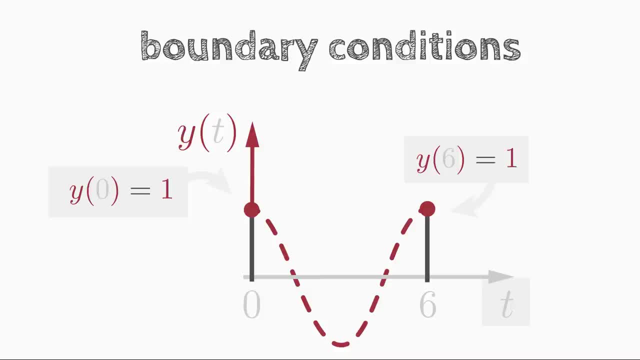 The sentence function values at two different points in time was, of course, just an example. Instead of time, it could be any variable that fixes the system at the boundaries At different times, at different positions, at different angles, and so on. So far, so good. Now let's look at four methods with which you can solve simple differential. 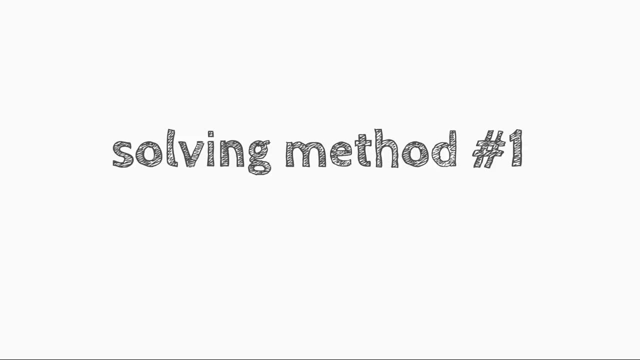 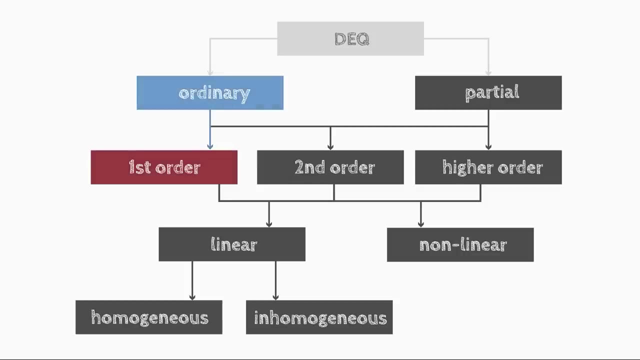 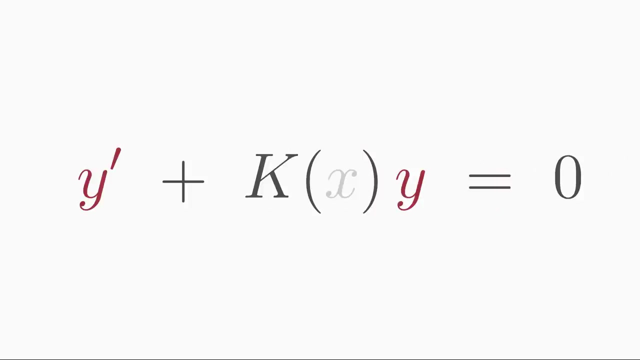 equations. Solving method number one: Separation of variables. With this method you can solve ordinary differential equations of first order, which must also be linear and homogeneous. This type of differential equations has the form y' plus k times y is equal to zero. The coefficient k must not necessarily be constant. 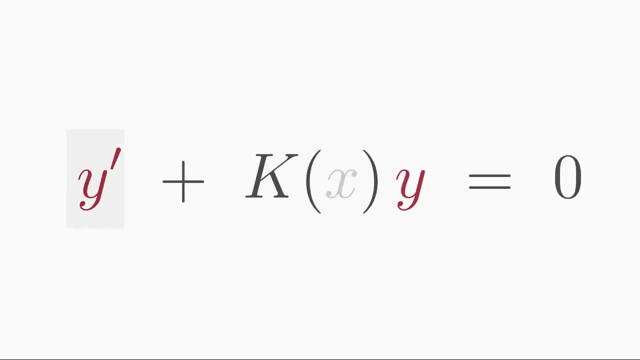 but can also depend on x. Also, note that before the first derivative, y', the coefficient must be equal to one. If this is not the case, then you simply have to divide the whole equation by the coefficient which is in front of y'. then you have the right form. 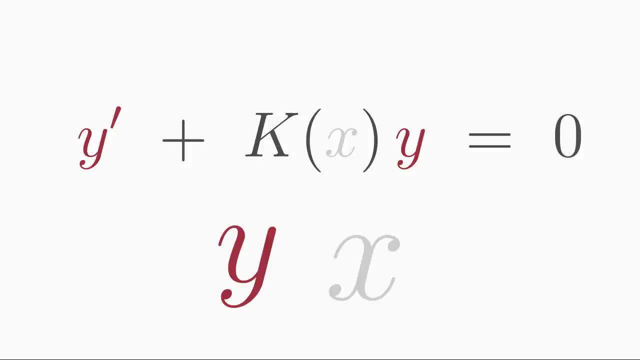 In this solving method, y and x are considered as two variables and separated from each other by bringing y to one side and x to the other side of the equation. The Leibniz notation of the differential equation is best understood by this method. 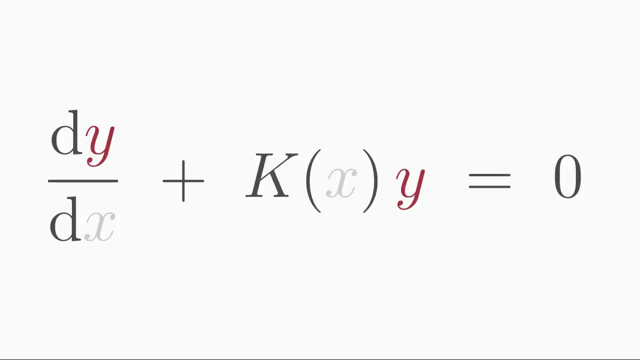 best suited for this purpose. Bring k times y to the right-hand side, Multiply the equation by dx and then divide the equation by y. This way you have only y-dependence on the left side and only x-dependence on the right side. Now you can integrate over y on the left-hand. 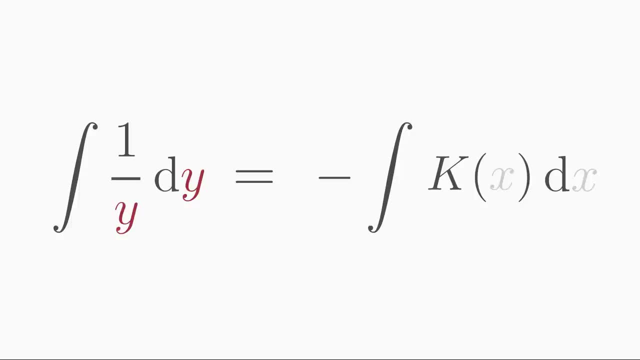 side and over x on the right-hand side. Integrating 1 over y gives the natural logarithm of y. Also, don't forget the integration constant. Let's call it a, for example. Now you have to solve for the function y. Use the exponential function on both sides. 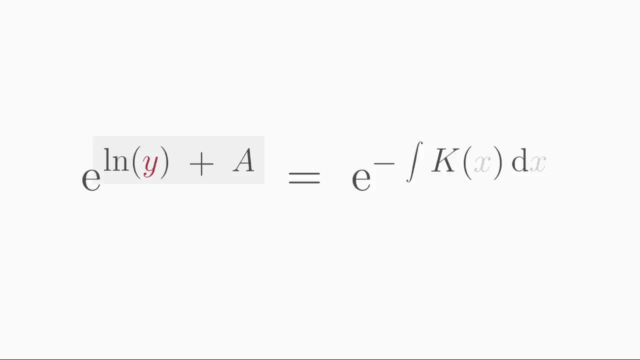 You can split the sum in the exponential term on the left side into a product where e to the power of ln of y is simple, Simply y. Bring the constant e to the power of a to the right side And rename the coefficient to a new constant c. As a result, you get a general solution formula that you can always. 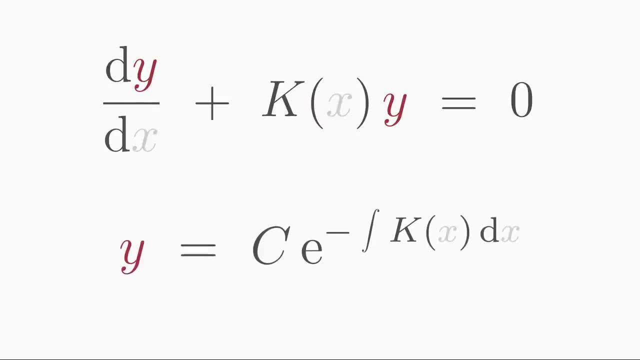 use to solve homogeneous differential equations. You don't have to apply the separation of variables method again and again, but you can use the solution formula directly. For example, let's look at the differential equation for the radial equation. In this case, the search function y is the number of not-yet-decayed atomic nuclei, n. 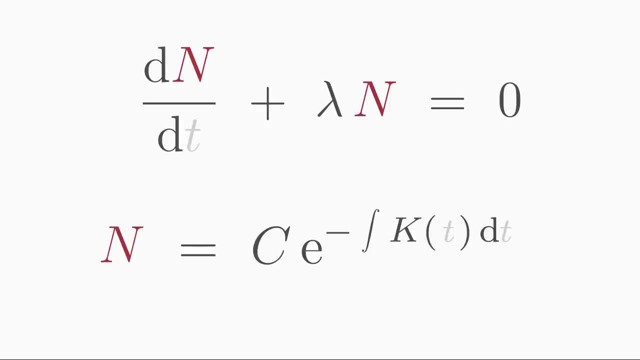 and the variable x corresponds to the time, t, And the coefficient k in this case is a decay constant lambda. According to the solution formula, you have to integrate the coefficient that is the decay constant lambda over t. Integrating a constant just gives t And we 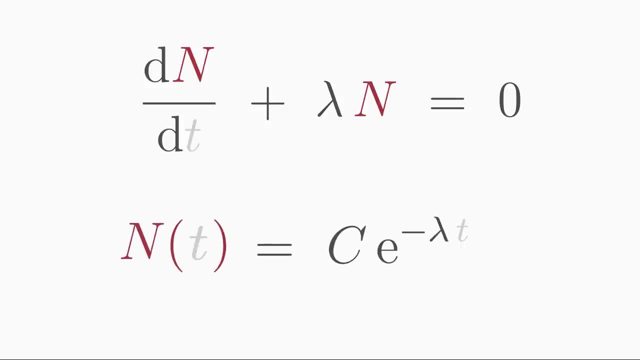 already have the solution formula. Now you know the qualitative behavior of the physical process, namely that atomic nuclei decay exponentially. But you cannot say concretely yet how many nuclei have already decayed after a certain period of time. This is because you don't know the constant c yet After. 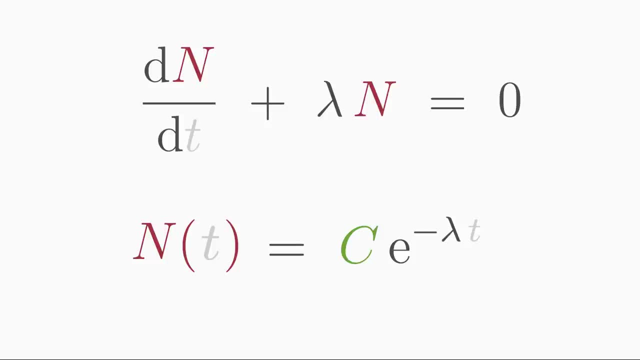 all in the decay law. c gives the number of atomic nuclei that are decayed after a certain period of time, not the number of atomic nuclei that are decayed after a certain period of time. You don't have to do that. The initial condition is to find the initial condition of the differential equation. 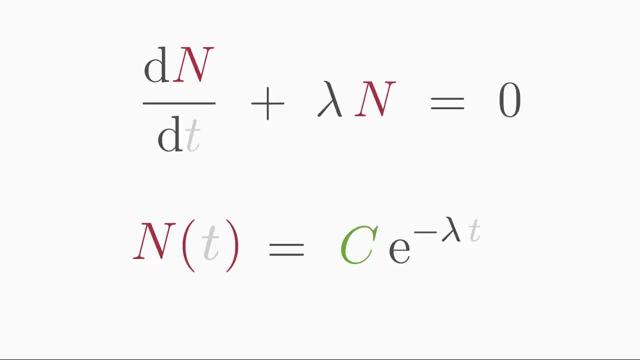 It could be, for example, like this: N of zero is equal to 1000.. That means at the time t equals zero. there were 1000 atomic nuclei. It could be, for example, like this: N of zero is equal to 1000. 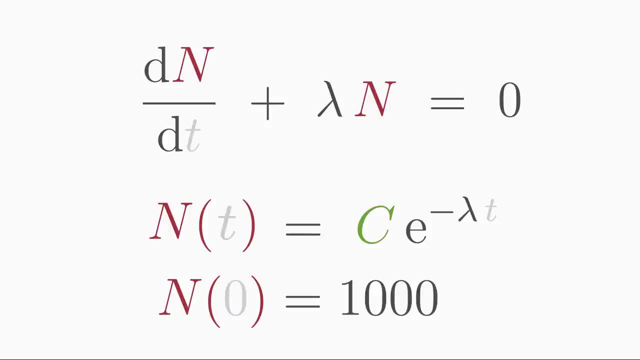 That means at the time t equals zero, there were 1000 atomic nuclei. Inserting this initial condition results in this equation: E to the power of zero is one, So c must be one, So c must be one be 1000. 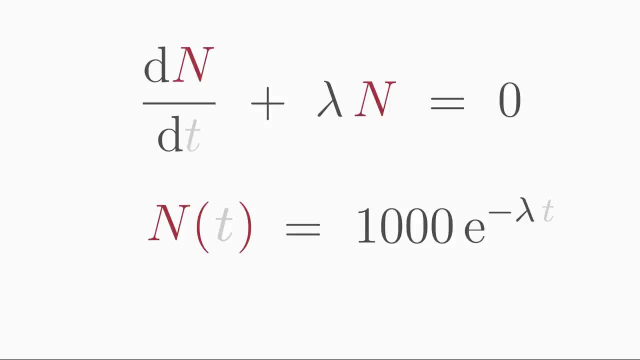 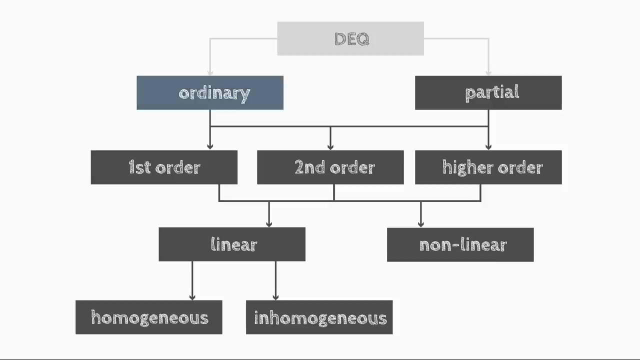 Now you can insert an arbitrary point of time and find out how many not-yet-decayed atomic nuclei are still there. Solving method number 2, variation of constants. This method is well suited for ordinary differential equations of first order which are linear. 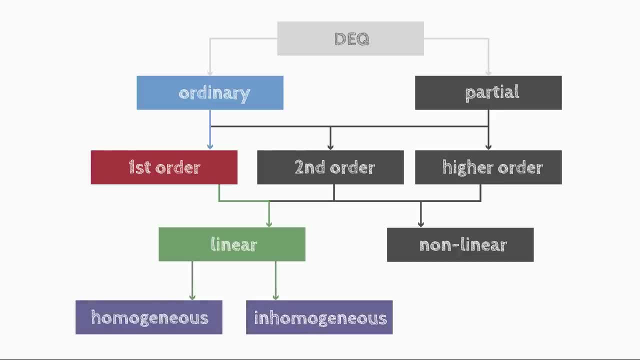 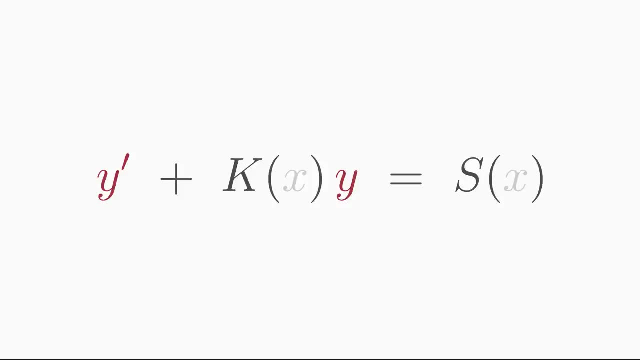 The differential equation can be homogeneous or inhomogeneous. The inhomogeneous one is more general. You have this type of differential equation. if you can bring your differential equation into the following form, y' plus k times y is equal to s. The inhomogeneous version differs from the homogeneous one only in the single coefficient. 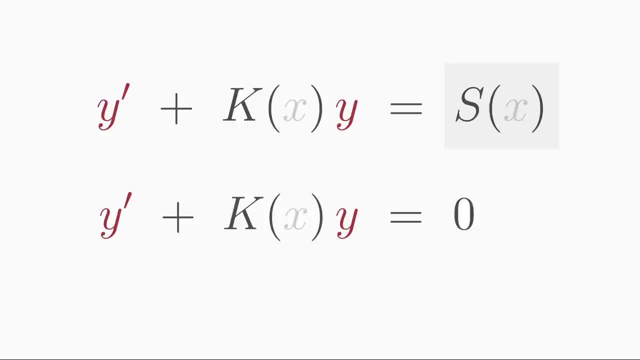 That is, the perturbation function s is not zero. Thus this type of differential equation is somewhat more difficult to solve. In this solving method you make the ansatz that the general solution y is given by a coefficient c that depends on x, multiplied by a homogeneous solution that we denote as: 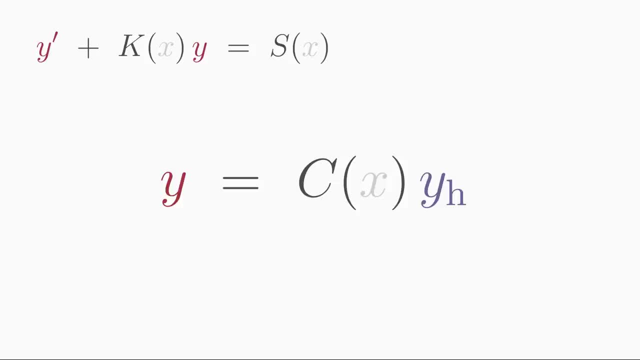 yh. You have already learned how to find the homogeneous solution yh with the previous method. All you have to do is to set the perturbation function. You have already learned how to find the homogeneous solution yh with the previous method. Then you have the homogeneous differential equation. 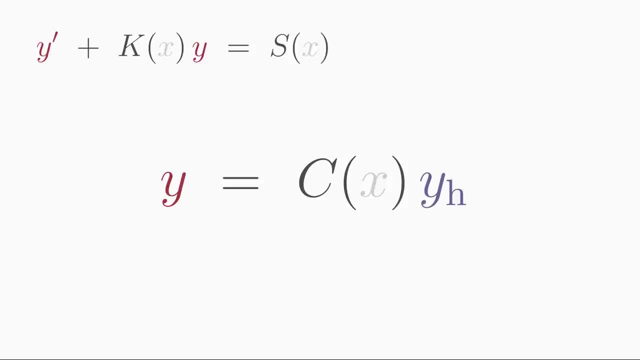 You solve it with the separation of variables method or directly by using the corresponding solution formula. Let us insert this ansatz into the inhomogeneous equation for y. We also want to replace the derivative y' with our ansatz. To do this, we must first differentiate y with respect to x. 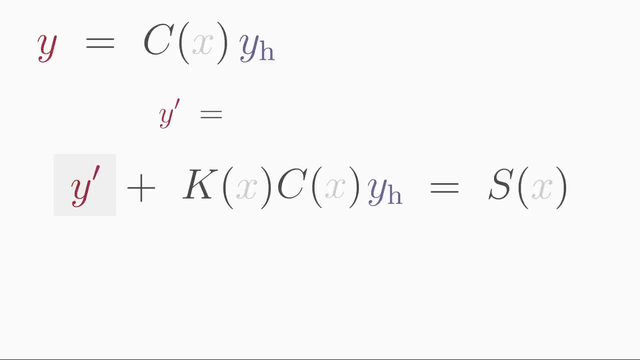 Since y is the derivative of y, we must first differentiate y with respect to x. Since both c and yh depend on x, we need to apply the product rule. You do this by differentiating c once leaving yh, and then leaving c and differentiate yh. 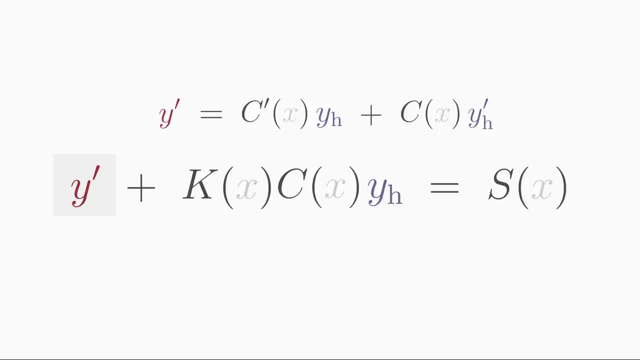 The result is the derivative of our ansatz. Now we insert the derivative y' into the inhomogeneous differential equation. If you just factor out c, you might see why this is a derivative of x and not of y, But this is still a derivative of y. 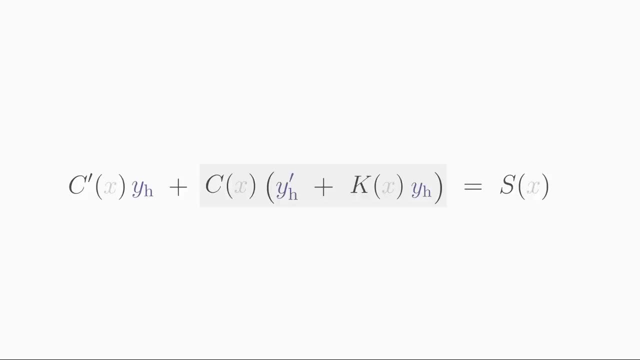 Now we insert the derivative y' into the inhomogeneous differential equation. If you just factor out c, you might see why this is a derivative of y. This approach is so awesome. In parentheses is the homogeneous differential equation, which is zero, so we can omit this. 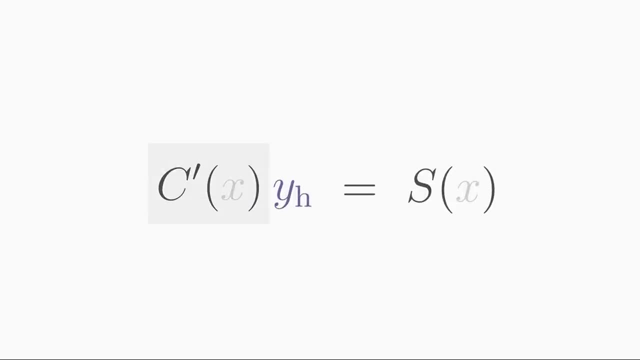 term completely. You can now rearrange the equation for the unknown coefficient c' Now, to eliminate the derivative c' we have to integrate both sides over x. We cannot integrate the right side concretely because s is different depending on the problem. 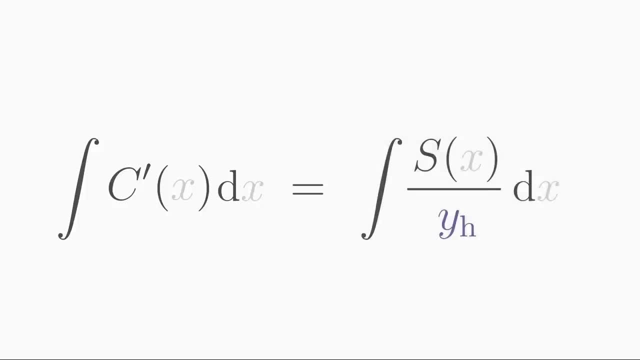 therefore, we leave the right side unchanged. The left side, on the other hand, can be integrated and additionally yields an integration constant. We put this constant directly on the right side and define it, for example, as a constant a. If you now just substitute the found coefficient c into the original ansatz, then you get the. 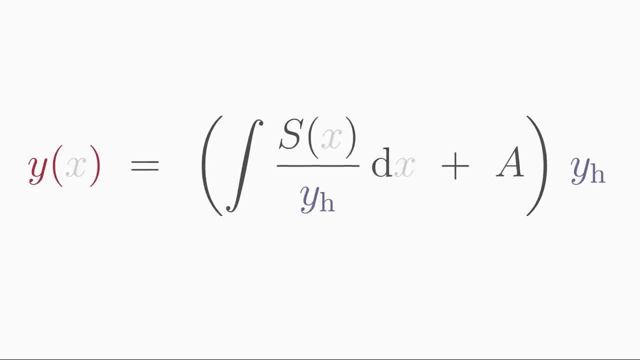 general solution of an ordinary linear differential equation of first order. Let's take an example from electrical engineering. Consider a circuit consisting of a coil characterized by the inductance L and a resistor R connected in series. Then we take a voltage source which provides a voltage u0, as soon as we close the circuit. 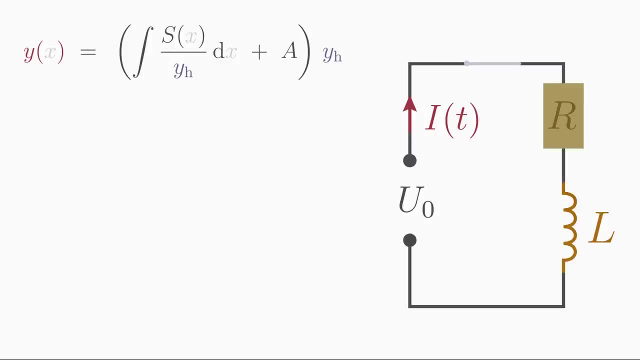 with a switch, Then a time-dependent current. I flows through the coil and the resistor. The current does not have its maximum value immediately, but increases slowly. Using Kirchhoff's laws, we can set up the following differential equation for the current I. 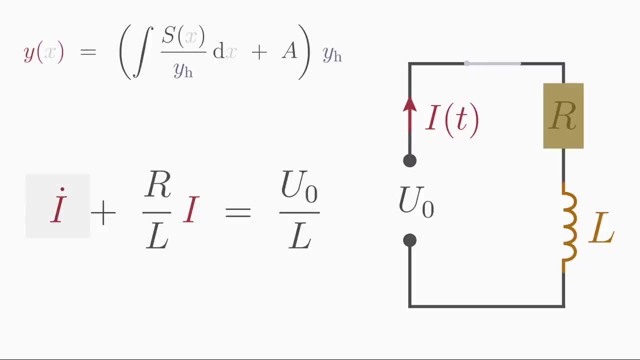 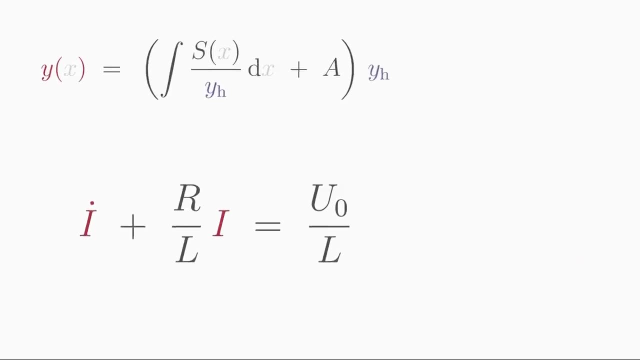 Remember that the point above the I means the first time derivative. This is an inhomogeneous linear differential equation of first order. The searched function y corresponds here to the current I. The perturbation function s corresponds to u0 over L, L and is time independent. in this case We denote the homogeneous solution by IH. 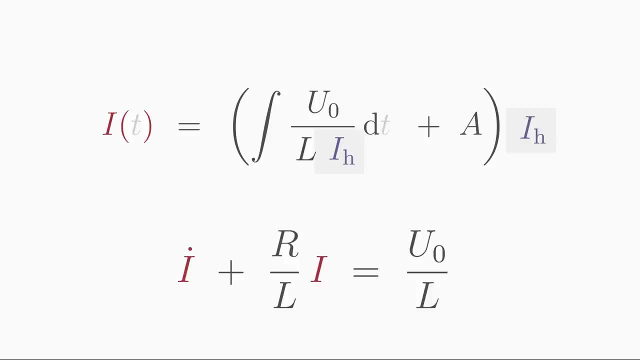 First we need to determine the homogeneous solution IH. We can quickly calculate this using the solution formula for the homogeneous version of the differential equation that you learned before. The coefficient k in front of the searched function i corresponds to R over L and is also time independent in this case. So far, so good. We may omit the constant CH in the 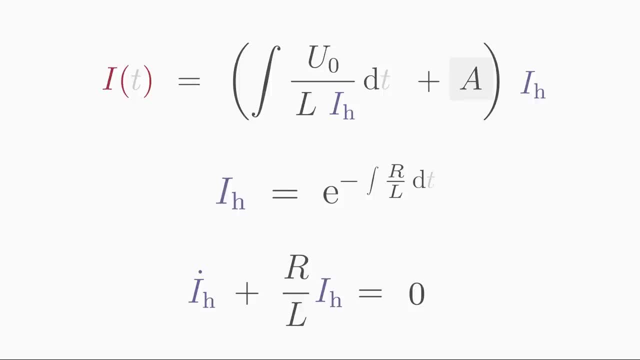 solution formula here, because we consider it later anyway. in the constant A which we find in the other solution formula, The coefficient R over L is constant, and integrating a constant only introduces a variable, t. Thus the homogeneous solution is: IH is equal to E to the power of minus. 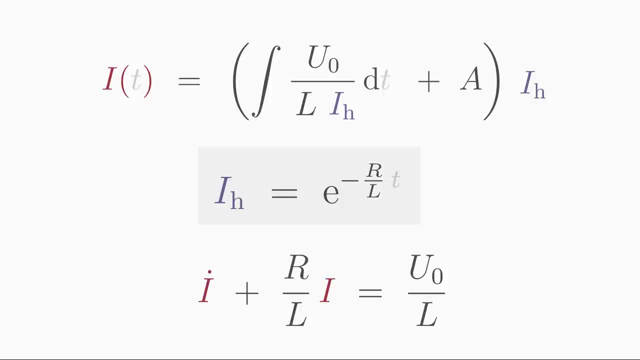 R over L. Let's insert it into the inhomogeneous solution formula. Note that 1 over the exponential function containing a minus in the exponent is simply equivalent to the exponential function without the minus sign. Now we have to calculate the integral. U0 over L is a constant and can be placed in front of. 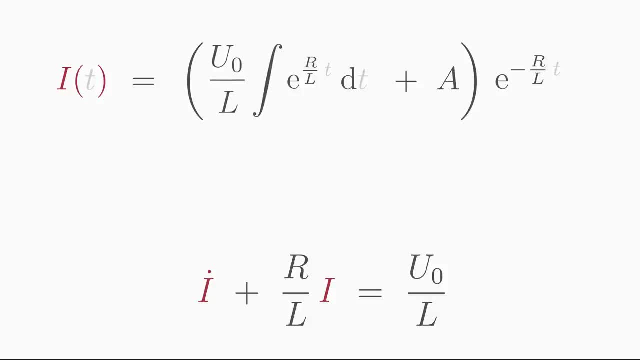 the integral And when integrating the exponential function, the exponential function is preserved. Only L over R is added as a factor in front of the exponential function. Finally, we hide the constant of integration in the constant A, And this is our general solution. We can simplify it a bit more by multiplying out the parentheses. 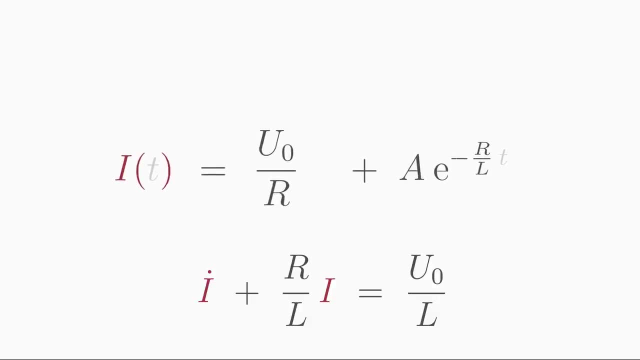 Two exponential functions simplify to one. To get a solution specific to the problem we need to determine the unknown constant A. For that we need an initial condition. If we say that the time t equals zero is the time when the current I was zero because we have not yet closed the switch, then our initial condition is Y of 0. 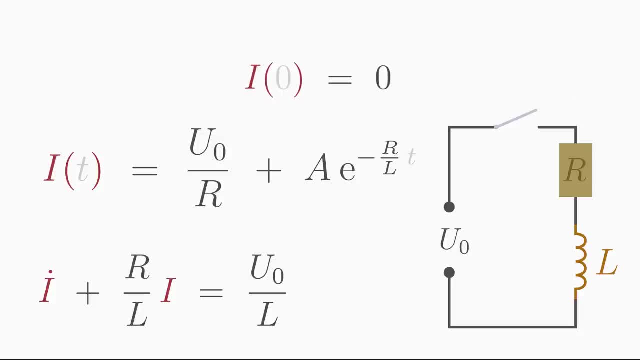 is equal to zero. Insert it into the general solution. E to the power of zero is equal to 1.. Solve for A and you get A is equal to minus U0 over R over L. Thus we have successfully determined the specific general solution. 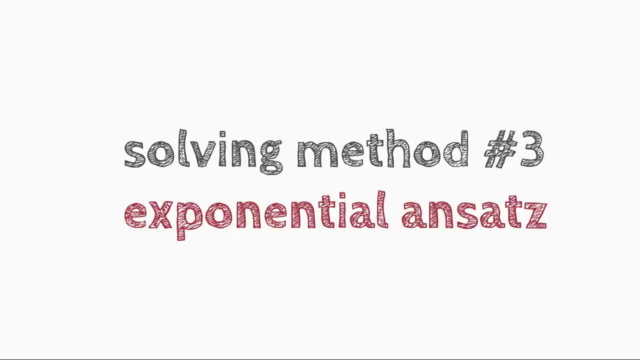 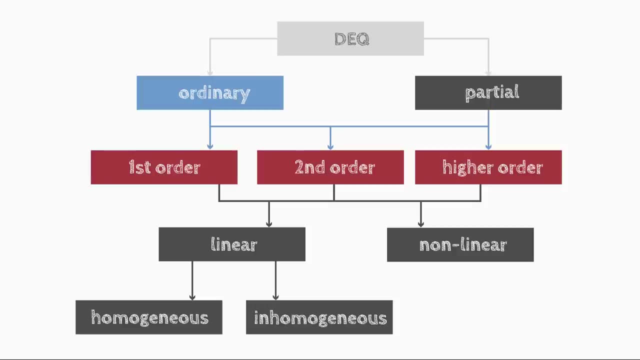 Solving method number 3.. Exponential ansatz. The exponential ansatz is suitable for ordinary differential equations of arbitrary order that are linear and have constant coefficients. Of course the method quickly becomes complex for higher orders The method is best suited for. 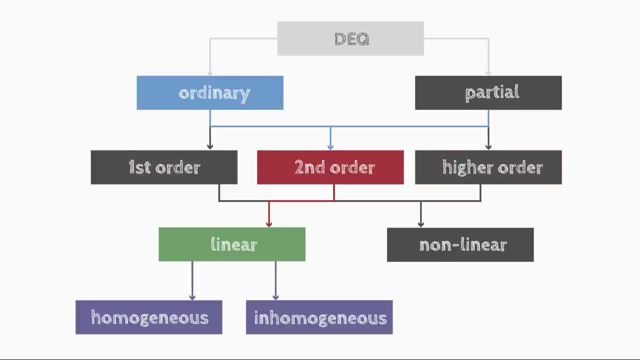 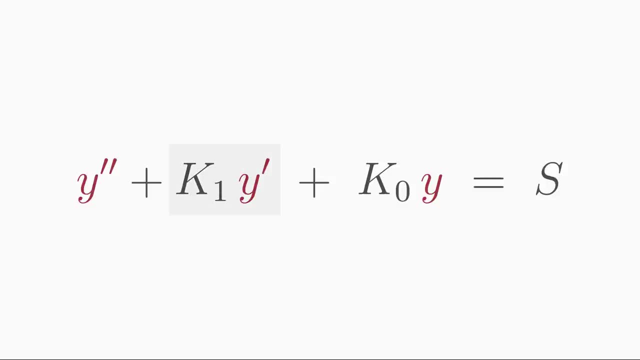 second-order differential equations. The general form of a second-order linear differential equation looks like this: Y'' plus K1 times Y' plus K0 times Y is equal to S. Here we assume that the coefficients K1 and K0, as well as the perturbation function S 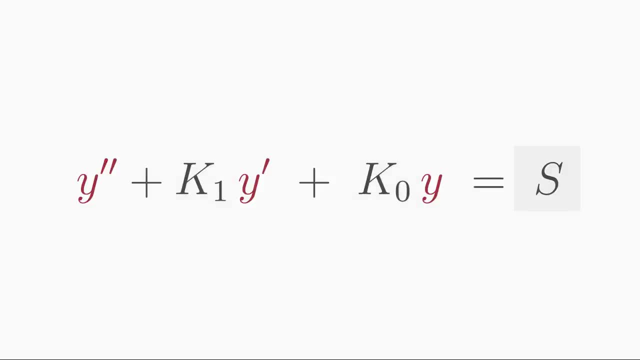 are independent of X, They are a constant. If the perturbation function is not zero, then you must first ask a mathematician. Then he will tell you that a general solution Y of an inhomogeneous linear differential equation is composed of two parts: A homogeneous solution YH of the homogeneous differential equation. 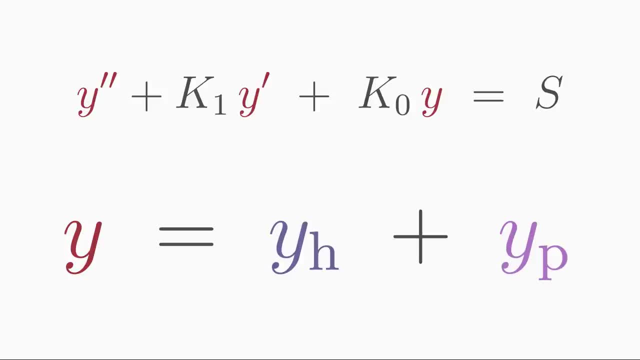 and of a particular solution which we denote by Yp. The homogeneous solution YH solves the differential equation. if you set the perturbation function S equal to zero, E to the power of zero is equal to zero. In the method of the differential equation, the perturbation function S is equal to zero. 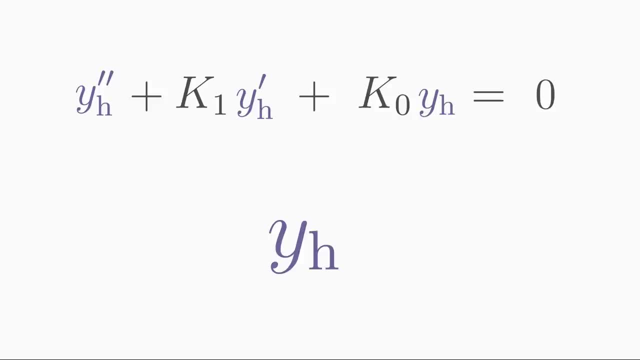 In the method of the exponential ansatz. as the name suggests, we make the guess that the homogeneous solution, YH, has the form of an exponential function. YH is equal to C times E, to the power of lambda times X, Since the first and second derivatives of YH occur in the general formula of the differential. 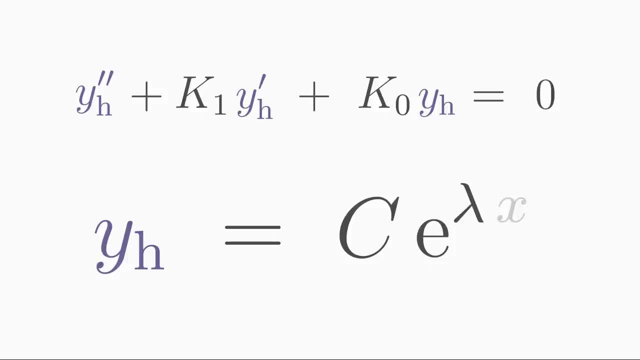 equation, we must differentiate our exponential ansatz twice. The first derivative is: YH' is equal to C times lambda times E to the power of lambda times X. And the second derivative is C times lambda squared times E to the power of lambda X. 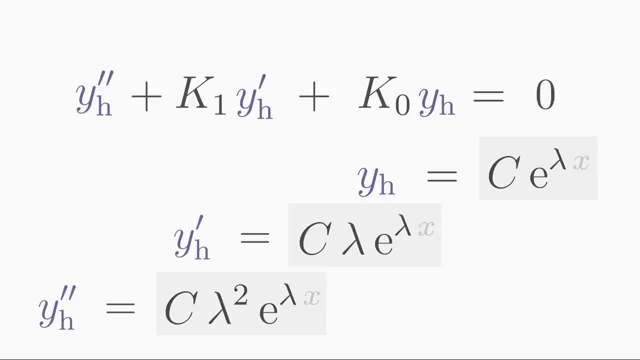 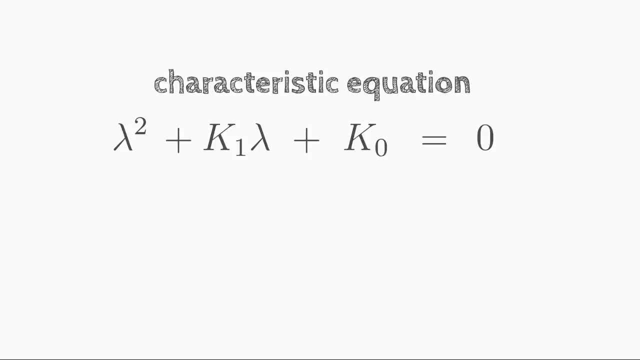 Now we can insert the exponential ansatz and the corresponding derivatives into the differential equation. Let us factor out C times E to the lambda X. If we divide by this factor, then we get C times E to the power of lambda X. Then we get the so-called characteristic equation for lambda. 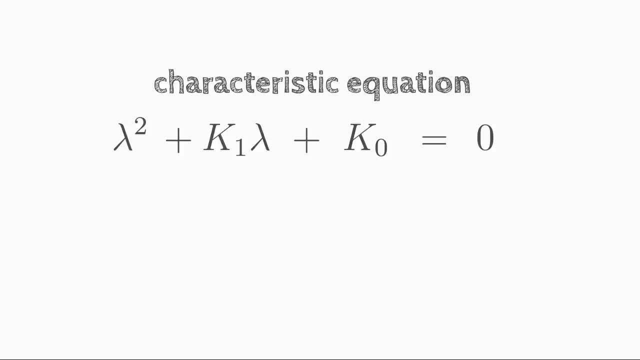 When we solve this equation, we find the unknown lambda. Since it is a quadratic equation for lambda, we get two solutions: Lambda 1 and lambda 2. We have to consider both of them. Basically, you can set up the characteristic equation directly by looking at your differential. 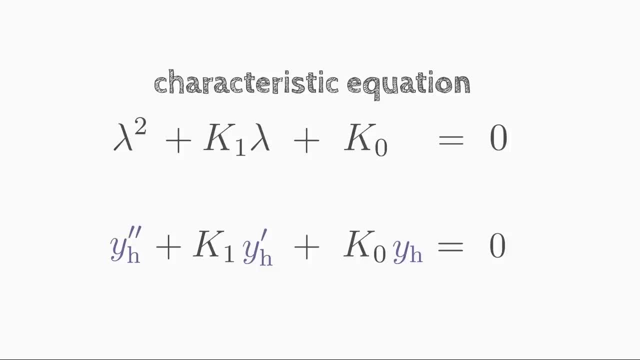 equation without having to do all these steps. Compare your differential equation with the characteristic equation. The coefficient in front of lambda squared is in front of the second derivative of Y. In this case, the coefficient is 1.. The coefficient of lambda is in front of the first derivative of Y. 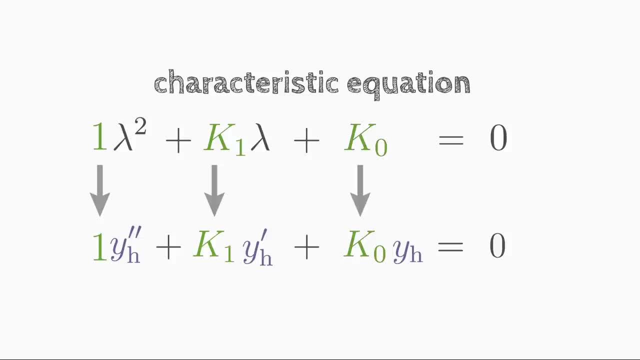 In this case K1.. And the coefficient K0 in front of the function Y itself stands alone in the characteristic equation. By the way, if you had a homogeneous third-order differential equation, then the characteristic equation would still be the same. It would start with the cubic term. 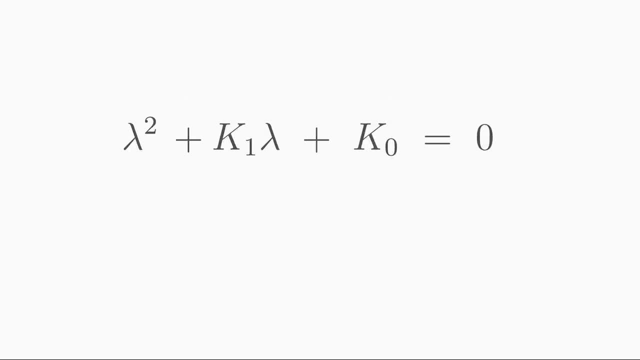 And so on. A quadratic equation has two solutions, lambda 1 and lambda 2.. And you can determine these, for example, with the quadratic formula. Since you get two lambda values, we have to consider both. To do this, you have to extend the exponential ansatz by another term. 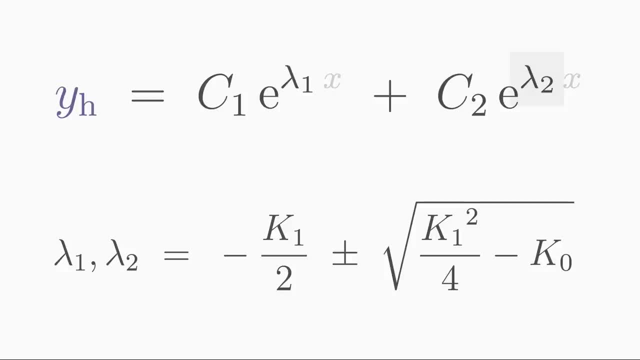 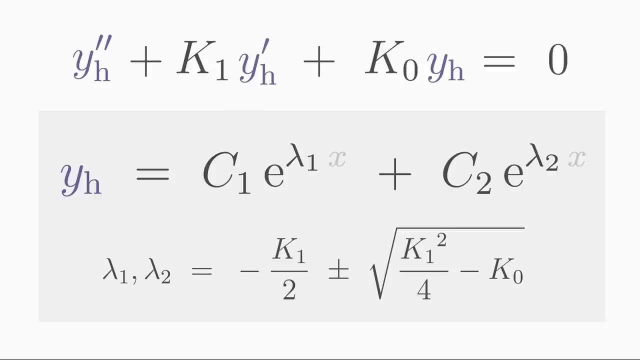 in which the second lambda value is in the exponent With the corresponding lambda values. this is the solution of the homogeneous term, And so on, If you have a homogeneous differential equation of second order depending on the values of the coefficients K1 and K0,. 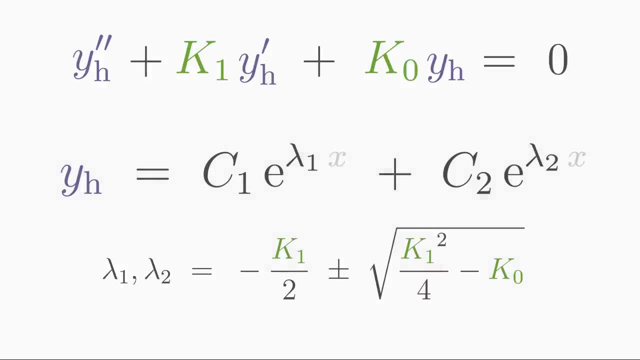 the solutions may show different behavior, Because if K0 is greater than K1 squared over 4, then you are taking the square root of a negative number. In this case, you get a solution that describes oscillations. I will show you this in an example. 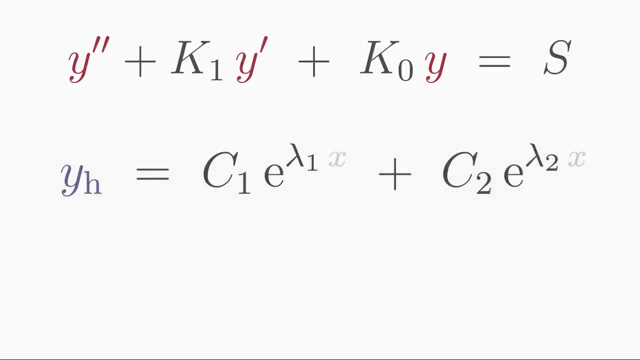 If the differential equation to be solved is inhomogeneous, that is, the perturbation function is not zero, then we still have to add the particular solution, yp, to the homogeneous one to find a general solution. For the particular solution, we have to choose an appropriate approach. 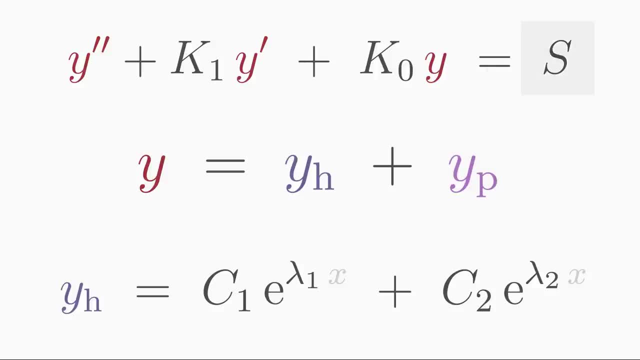 depending on what form the perturbation function s has. Here we look at the simplest possible form, namely when the perturbation function s is constant, Then the particular solution is given by a perturbation function divided by the coefficient K0.. yp is equal to s over K0.. 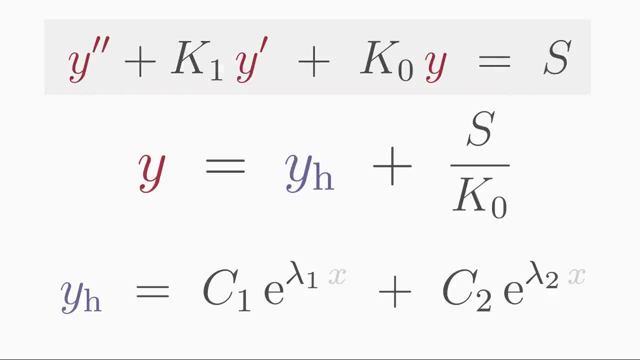 Now, to get a general solution of such an inhomogeneous differential equation, we have to add the homogeneous solution and the particular solution. The two unknown constants- C1 and C2, are determined by the constraints, as you know. Also note that this method of the exponential ansatz is a guess method. 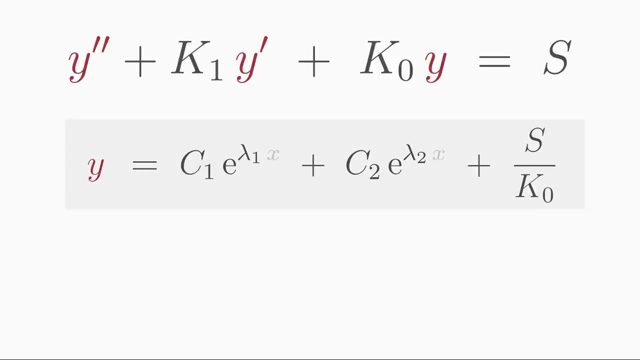 this is the case if the actual solution of the differential equation is not of exponential form. Therefore, if you use a solving method that contains the word ansatz in its name, be sure to check your solution. You do this by substituting the solution you have found. 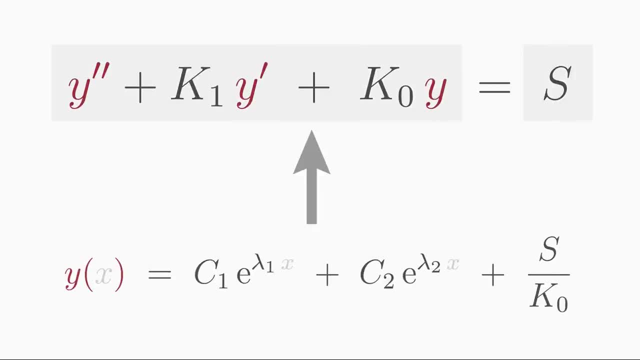 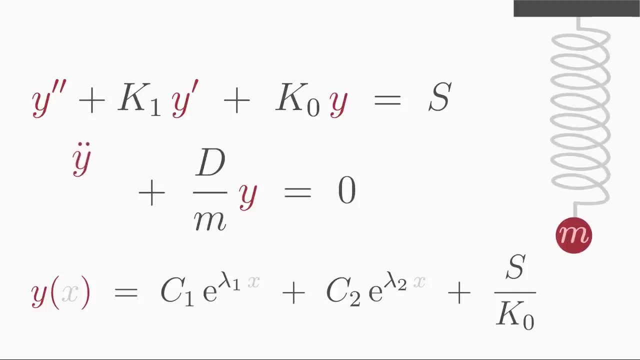 in the differential equation and checking if both sides are equal. Let's make an example. Do you remember the differential equation for the oscillating mass? This is a second-order differential equation with constant coefficients. The perturbation function is 0. That means we only have to find out the homogeneous solution. 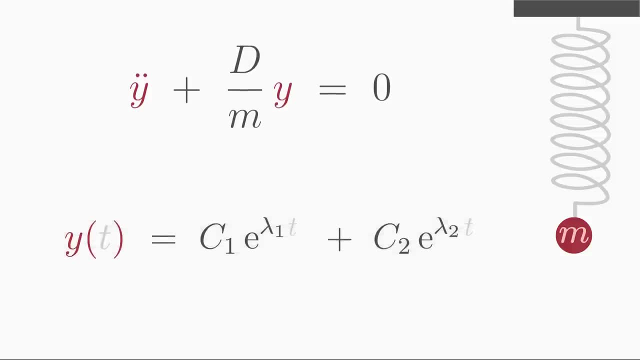 And we do that with the exponential ansatz we just learned. Let's take the FAST way and directly write down the characteristic equation. We expect a quadratic equation because we have a second-order differential equation equation. The second derivative is preceded by the coefficient 1, so we just write lambda. 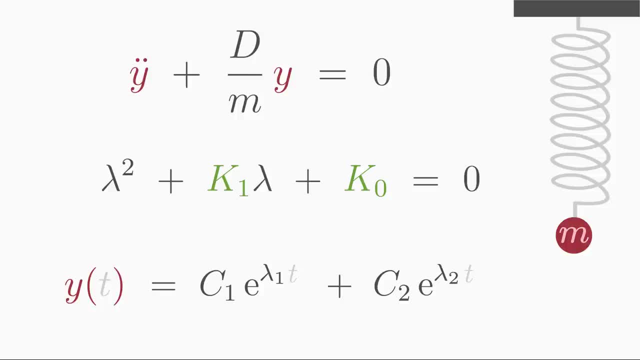 squared, Then the coefficient in front of the first derivative. Since the first derivative is missing in the differential equation, the lambda term is absent as well. Next up is the coefficient d over m, that is, in front of the searched function. This coefficient stands alone in the characteristic equation Altogether. the characteristic equation reads: 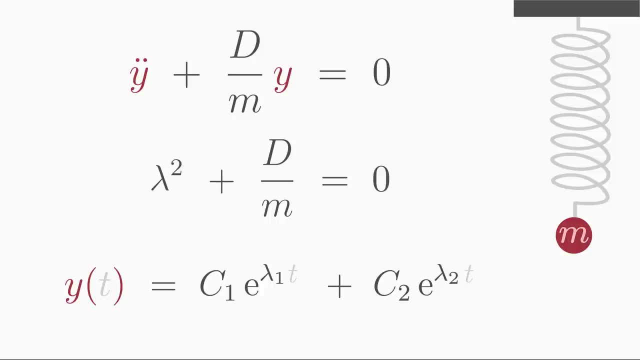 lambda, squared plus d over m is equal to zero. For this equation we don't even need the quadratic formula. We get the solution directly if we first bring d over m to the other side and then take the square root. Consider that the inverse of squaring gives two solutions: a positive and a negative square root Also. 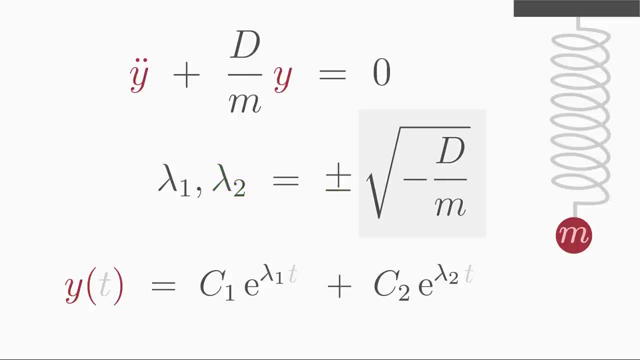 we have an interesting case here when the square root of a negative number is taken. Square root of a negative number is not a real number, but an imaginary number. Do you remember what that means? We expect that the system must oscillate, Even if you don't. 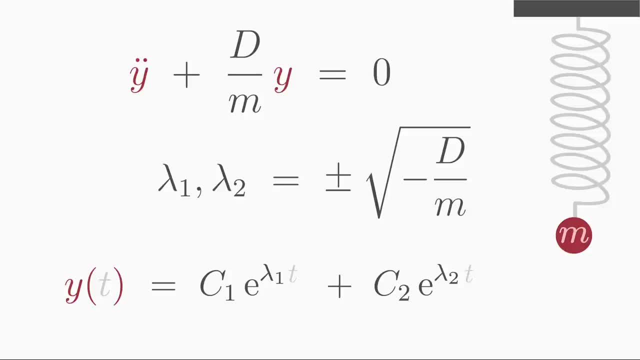 know imaginary or complex numbers. yet you can split the term inside the square root into a product of minus 1 and d over m. According to the square root laws, you can split this product into two square roots. Square root of minus 1 is defined as the product of minus 1 divided by d over m Square root. 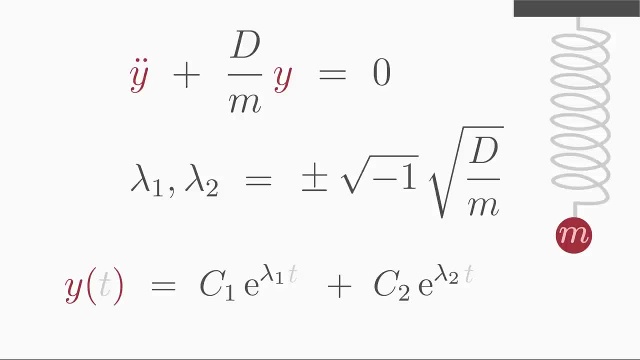 of minus 1 is defined as the product of minus 1 divided by d over m. Square root of minus 1 is defined as the imaginary unit, a number which we denote by the letter i. That's all you need to know about imaginary numbers. Let us denote square root of d over m shortly. 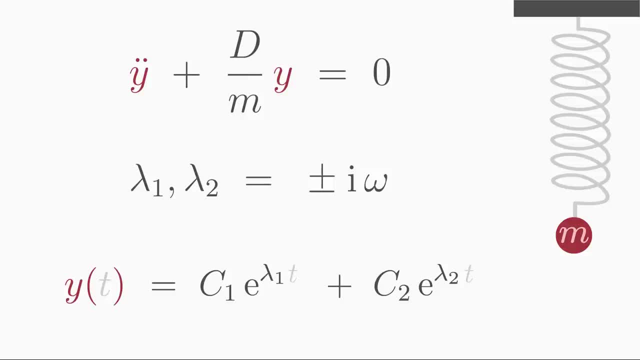 as omega. If we insert the lambda values we have just found into the exponential ansatz, we get the general solution for the considered differential equation. This solution seems very abstract, but I will show you that this solution can respond to an oscillation. Before that, let us determine the unknown. 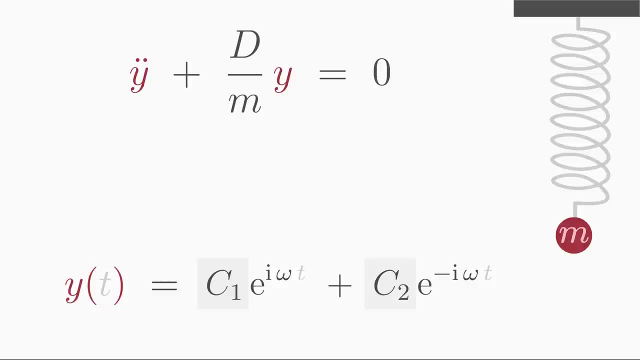 constants c1 and c2 with initial conditions for our problem, For example, we could have observed that at the time t equals 0, the displacement of the spring was 1.. The spring was displaced to the maximum, so the initial condition is y. 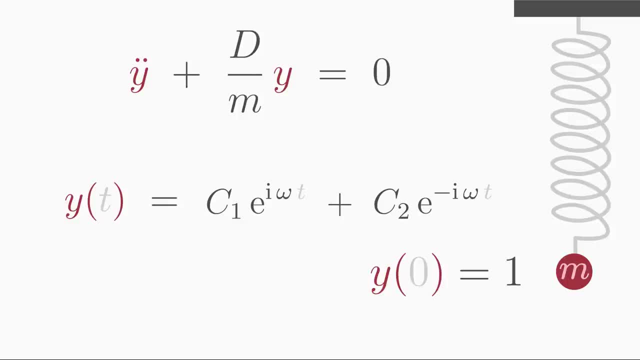 of 0 is equal to 1.. Insert this condition into the solution to determine c1.. e to the power of 0 is 1.. Rearrange for c1 and you get c1 is equal to 1 minus c2.. Next step is to determine the unknown constant c2 using the second initial condition For. 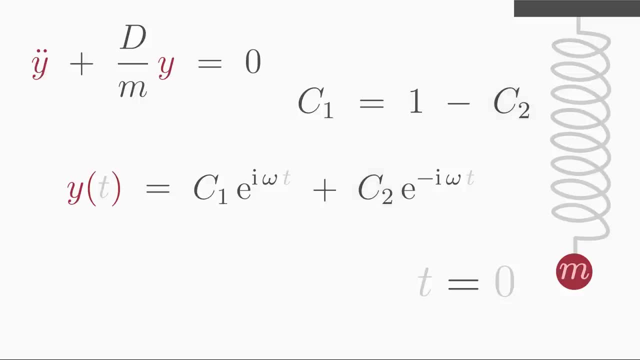 this we use the fact that at t equals 0, the velocity of the mass was 0. In physics you learn that velocity corresponds to the first time derivative of the displacement. For example, at t equals 1.. So our second initial condition is given by y, prime of 0 is equal to 0.. 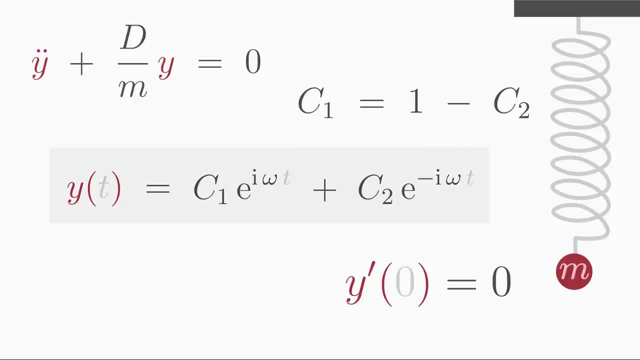 So let's differentiate our general solution with respect to time t. The factor in front of t becomes a factor in front of the exponential function, And then we insert the second initial condition into the derivative. The exponential functions become 1 and the factor i omega. 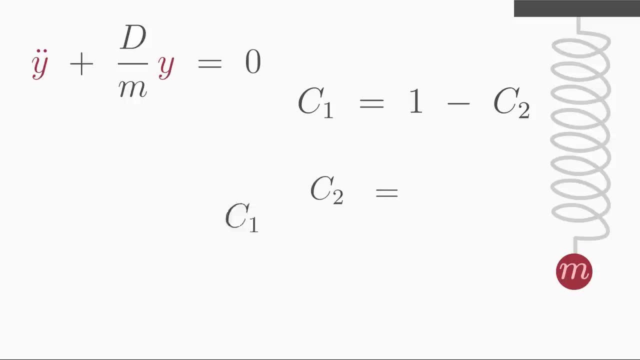 cancels out For c2, we find out that c2 is equal to c1.. So we know that c2 must be equal to c1.. Nice, Let's replace c2 with c1 to determine concrete value for the constants. The equation results: 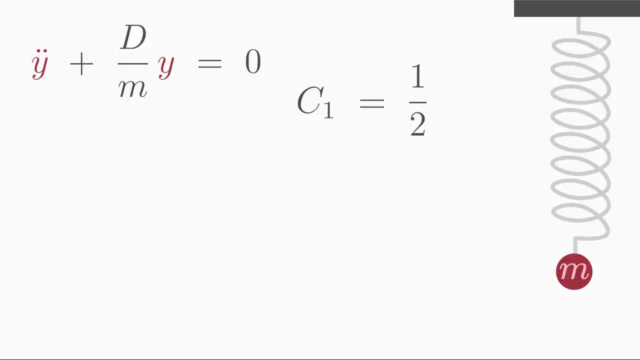 in c1 is equal to 1 half. Since c1 and c2 are equal, c2 must be also equal to 1 half. Insert 1 half into our general solution. Now let's find out what this abstract solution has to do with oscillations. For this we get: 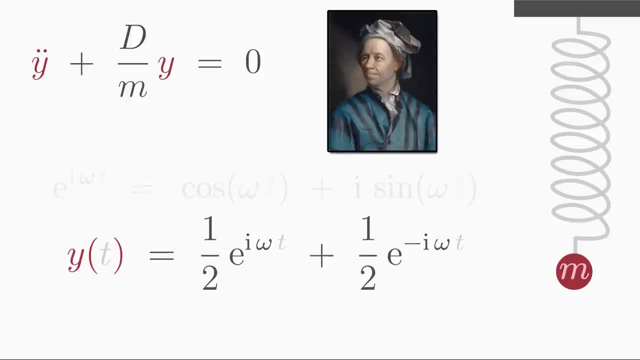 our friend Euler to help us, who tells us his famous Euler formula: e to the power of i, omega t is equal to cosine of omega t plus i times sine of omega t. This relation tells us how the complex exponential function is related to cosine and sine functions. So the 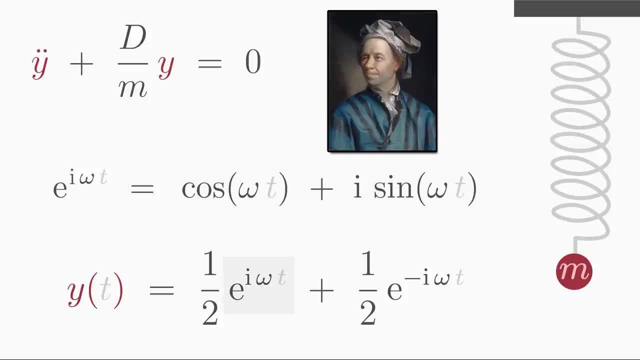 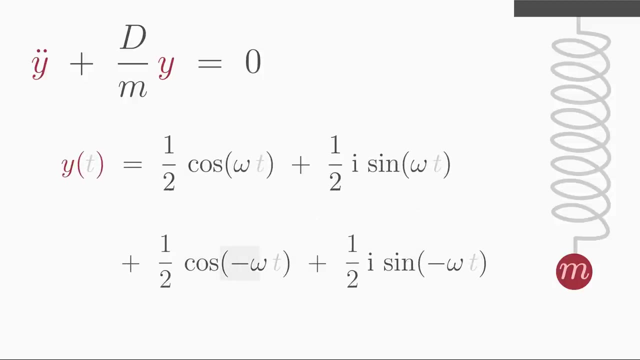 first complex exponential in our solution becomes cosine and sine with positive omega t, and the second complex exponential becomes cosine and sine with negative omega t. We can omit the minus sign in the argument of the cosine function because cosine is symmetric. That means it has the same value for arguments x and minus x, The sine function. on the argument. 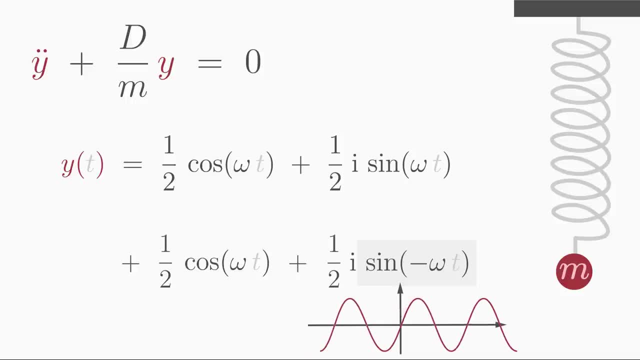 on the other hand, is anti-symmetric. Therefore, we cannot omit the minus sign in the argument, but rather pull it out in front of the sine function. Very nice, The complex sine function drops out And the cosine can be summed up. 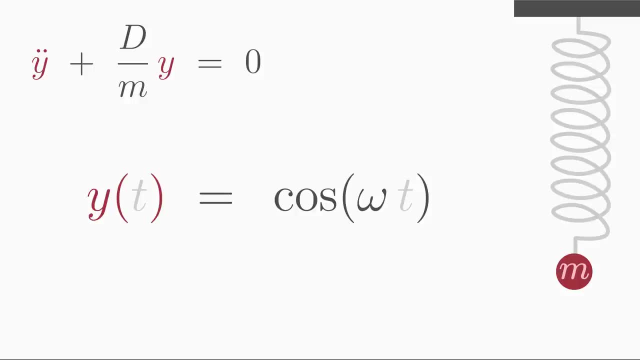 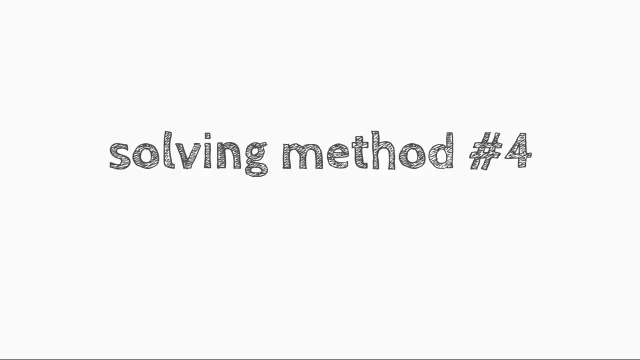 And this is our final solution. As you can see, the displacement y changes periodically with time. The mass attached to the spring oscillates back and forth and the oscillation is described by the cosine function. Solving method number four: Separation ansatz. This is sometimes called the product ansatz. 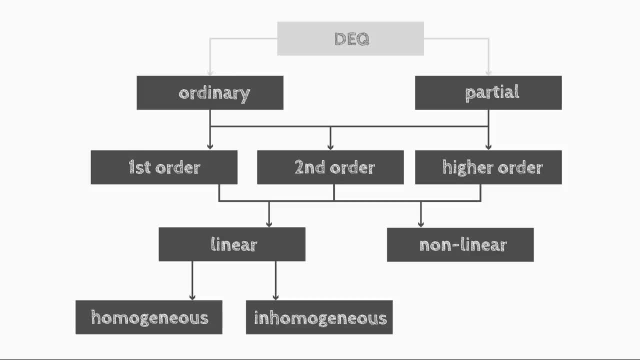 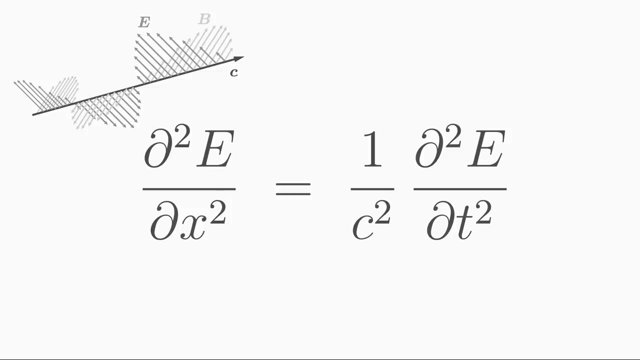 for reasons we will soon understand, This method is suitable for partial differential equations of arbitrary order. This solving method is only used to transform a partial differential equation into several ordinary differential equations and then to solve them with other methods. Let us illustrate this method directly with an example. Let's take a look at the one-dimensional. 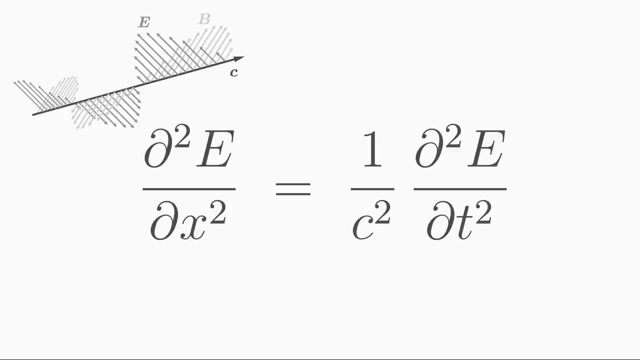 wave equation for an electric field. The function we are looking for is the electric field E. This depends on the position x and on the time t. Since the function depends on two variables and their derivatives appear in the equation, it is a partial differential. 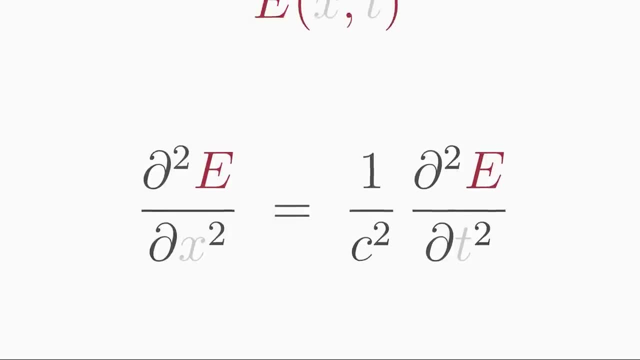 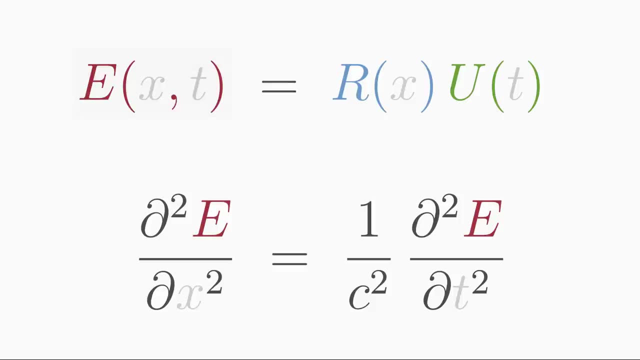 equation. Here we make a product ansatz for the searched solution E. e is equal to r times u. We assume that the solution e can be split into a product of two functions that we call r and u. One function, r, depends only on x and the other function, u, depends only on t. 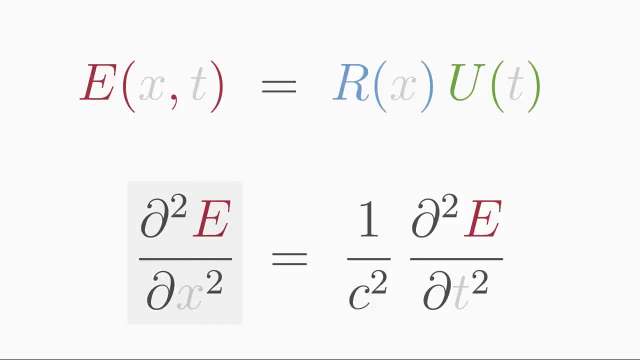 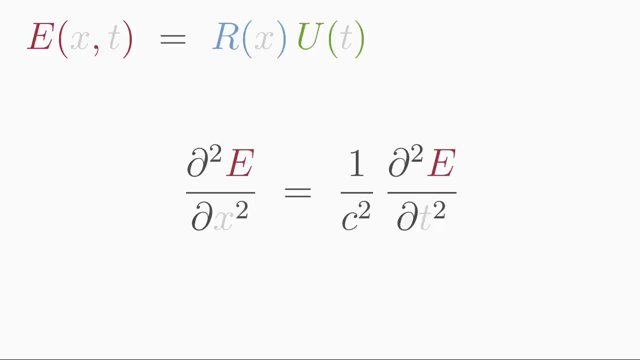 In the wave equation we have a second derivative of e with respect to location x and a second derivative with respect to time t, Differentiating the product ansatz with respect to x yields u times. the second derivative of r with respect to x, since u is independent of x and thus acts like a constant. 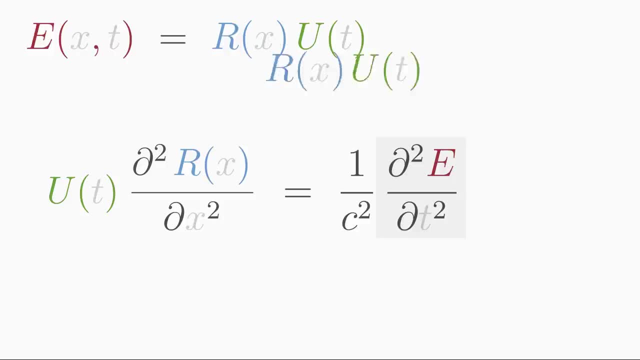 In contrast, in the derivative of the product, with respect to time t, the function r acts like a constant because it does not depend on t. The goal now is to separate everything that depends on x from what depends on t. Thank you. 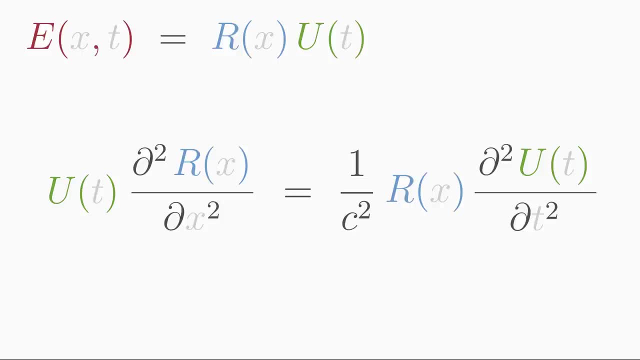 For this we divide this equation by r times u. Thus we have achieved that everything that depends on x is on the left side and everything that depends on t is on the right side. If you managed to separate a partial differential equation this way, then the separation ansatz 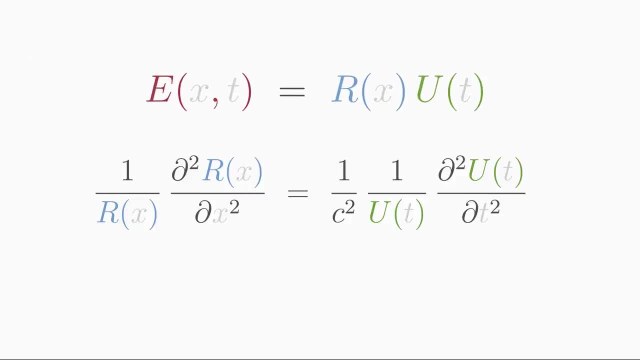 was successful. Now we can vary x on the left side without changing the right side. We will marry a differential equation on the right side because there is no今 on the right side. The same is true for the time t. If we vary the time on the right side, the left side remains unchanged because there